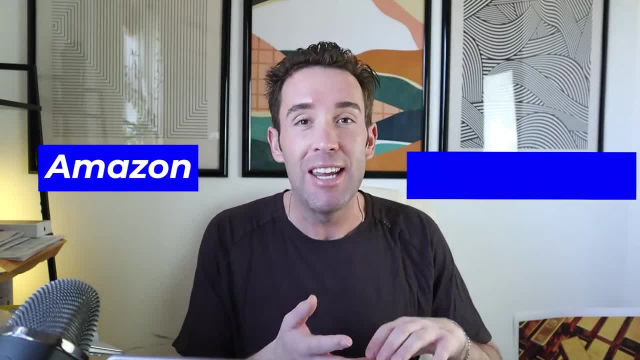 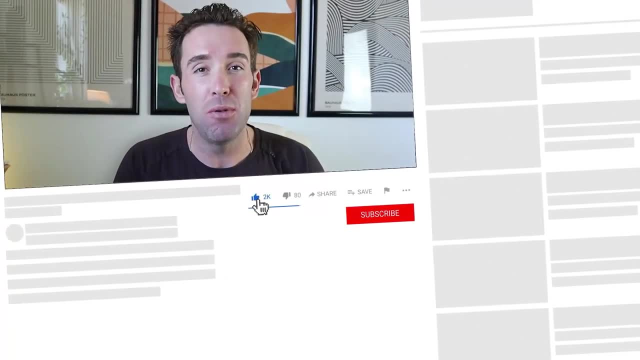 on this YouTube channel. I release monthly videos covering everything: Amazon, e-commerce and personal development. If you enjoy those types of videos, do me a favor right now: Head on down and press subscribe. I can see each and every one of you who take just a. 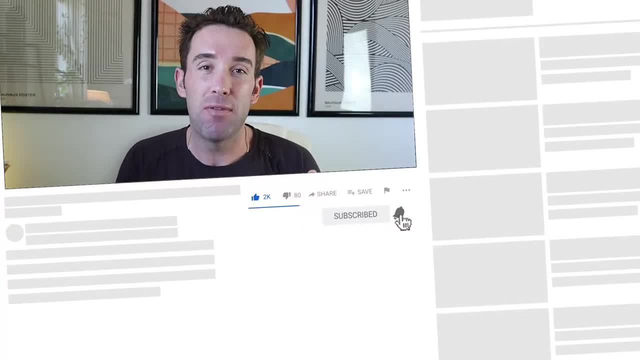 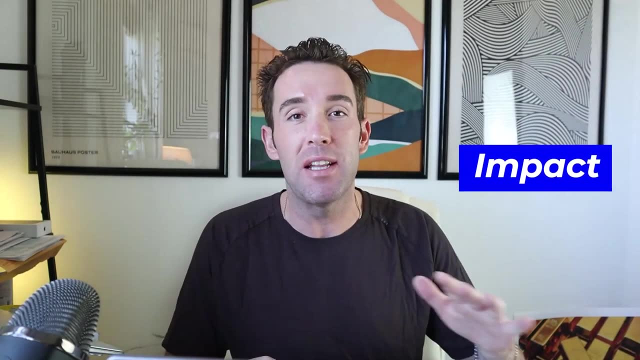 minute to press subscribe and I appreciate each of you Also give me a like on this video. It helps support my channel and bring you more helpful videos like this one. My job right here is to help educate, teach, impact as many lives as possible, sharing. 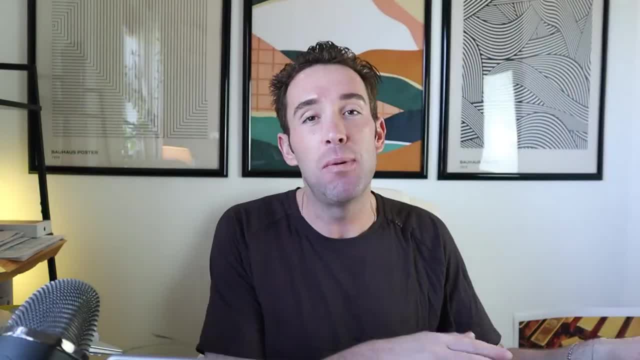 and documenting the world. I'm Brian Newton. I'm a full-time Amazon FBA seller. mentor my journey of how I went from a struggling broke drug addict to building multiple six-figure online businesses. Let's jump into it Up. first, let me just kind of go over. 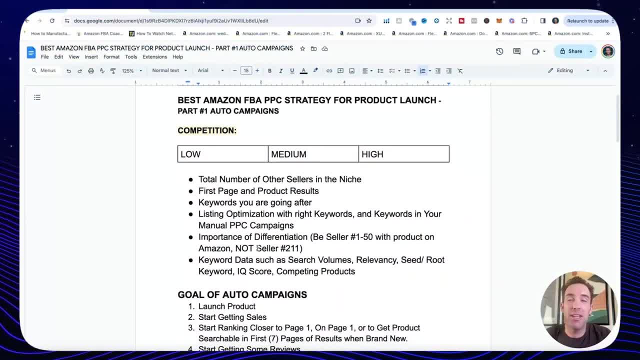 is it essential to set up Amazon PPC campaigns? Do you still need to run them? The answer is yes, guys. Amazon's more competitive than ever. It's going to be essential that we're setting up PPC different types of campaigns, including automatic campaigns, manual, keyword campaigns. 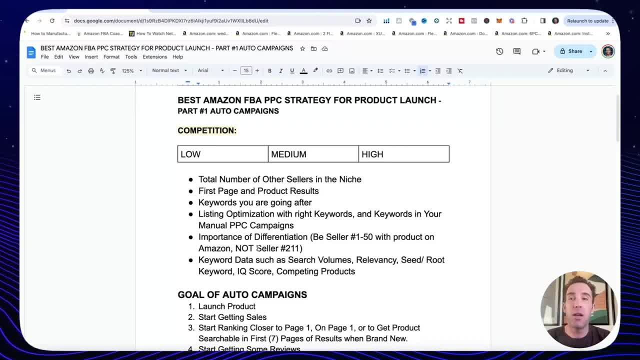 and product targeting campaigns to really push your product into the market, to start ranking for your main keywords, getting reviews, and to really push your product into the market. So in this video today, I'm going to be going over what types of campaigns to set up for new 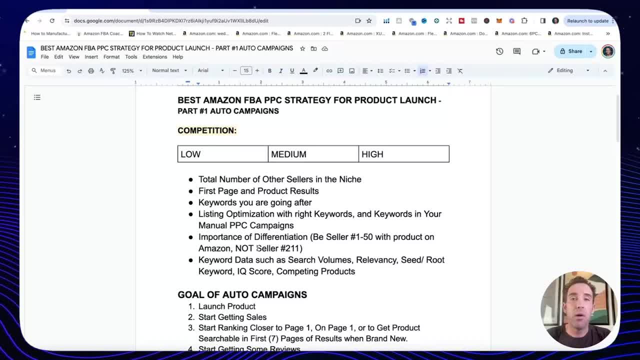 product launches, what to set for your budgets, your bids, what types of keywords to target, what types of campaigns to set up, how long you keep them running. all of that All right, so let's go over first: when do you set up these campaigns and what do you need in order to set up? 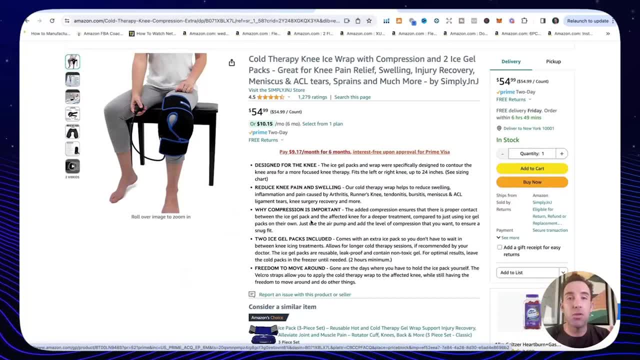 the campaigns themselves. So I recommend setting up your campaigns, most of these campaigns, all the auto ones- I'm going to show you the manual keyword ones and the product targeting campaigns- from day one of launch. I would wait until you had a couple. reviews only on like the exact match campaigns. For all the other campaigns, guys, we're going to be setting up 8 to 15, 8 to 15 different campaigns for a new product launch. I would set all those up from day one. So we're going to set up campaigns as soon as your listing status. 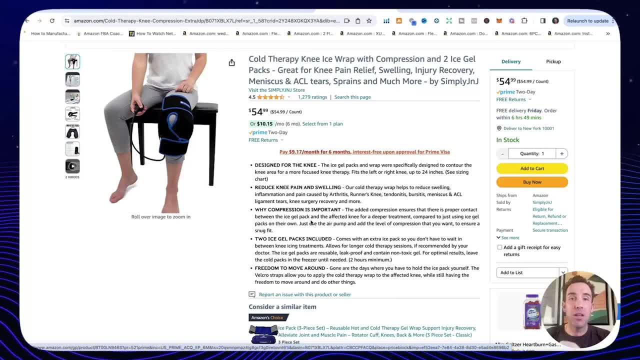 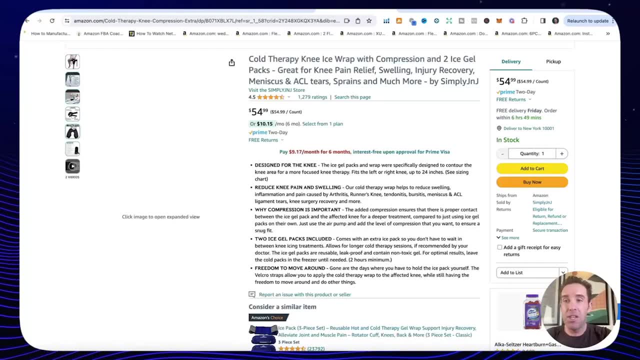 goes active. You have at least 50 to 100 units available and checked in at the Amazon warehouse and your listing is completely ready. You've uploaded all your images. You've got a really optimized, good title. You've got really good bullet points, five really good bullet points. 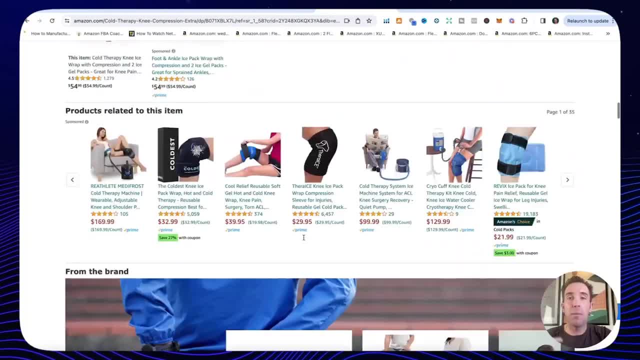 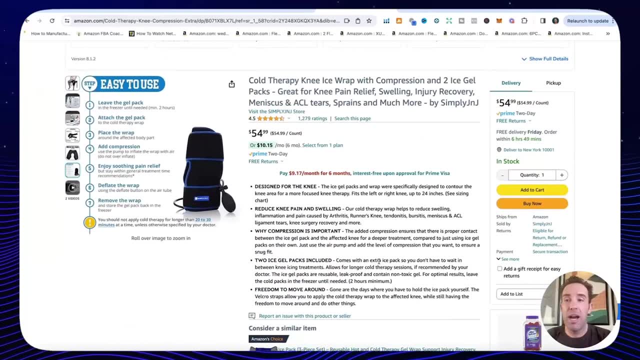 some selling features. You've done your description. You've optimized the back end with good keywords, You're going to be completely ready to go. If you're not at that stage yet where you haven't optimized your listing or you need help finding the best keywords to put in your 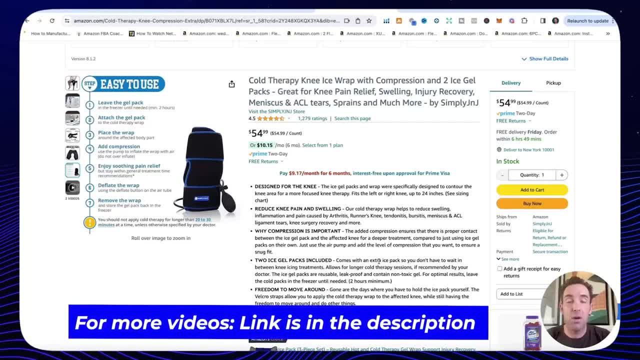 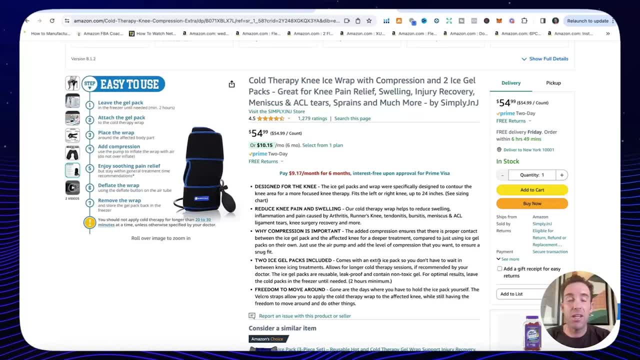 listing and for PPC. I have some other videos on my channel where I talk about how to do that. I will try to link those down below or there'll be a pop-up that comes up above where you can go and check out how to create your listing, how to find the best keywords and how to optimize your. 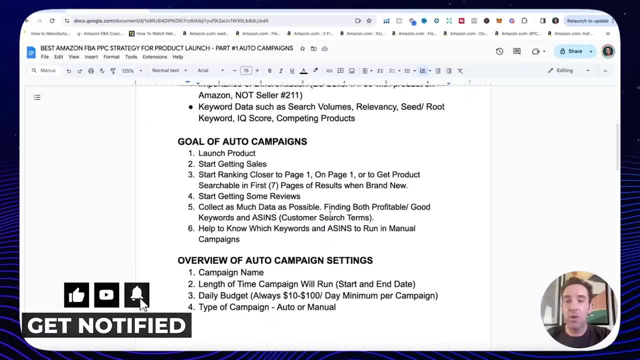 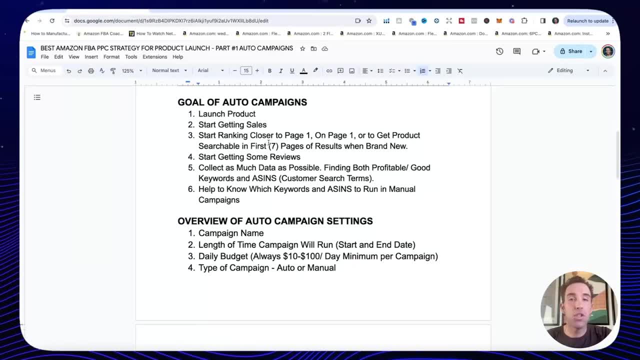 listing. Okay, so let's go over what I'm going to be showing you today. So the goal of campaigns, really both auto and manual, are going to be to launch the product, to start getting sales, to start ranking in the first seven pages of results. The truth is your product and listing. 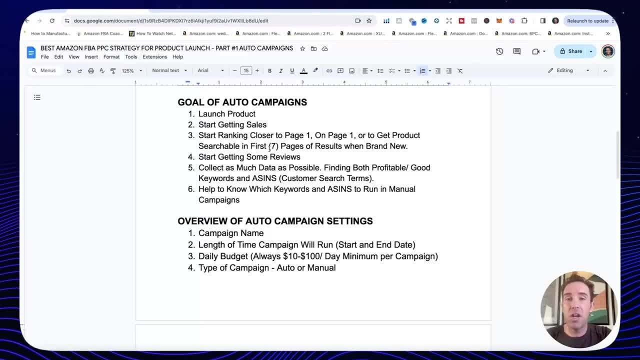 probably you will not be able to find it for more competitive niches First seven pages, even after your listing is live. So don't freak out if you can't find your product. As long as your listing says active and you've got units available, you are live. 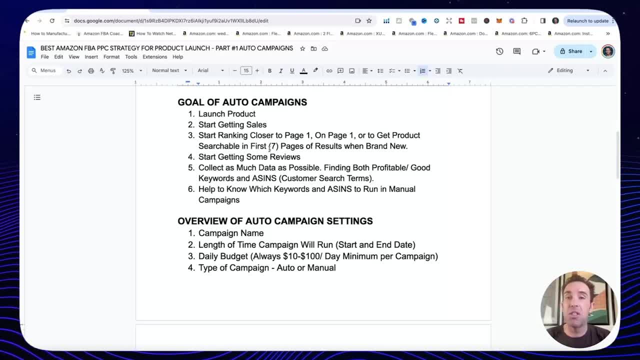 But typically Amazon won't show you in the first seven pages of results until you've made a couple sales. So that's why it's even more important that we turn on these PPC campaigns So you start getting sales, You start getting shown in the first seven pages and where you want to start, 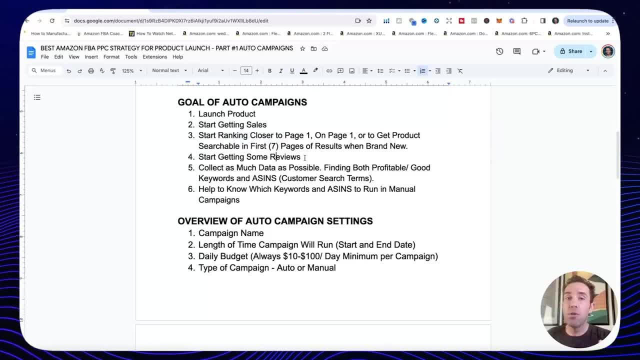 getting some reviews from the sales that we make. Reviews are going to help you get more sales Ranking and these PPC campaigns perform better, And we want to collect as much data as possible. So, yes, it sounds like a lot. We're setting up eight to 15 different campaigns. Each one is going to 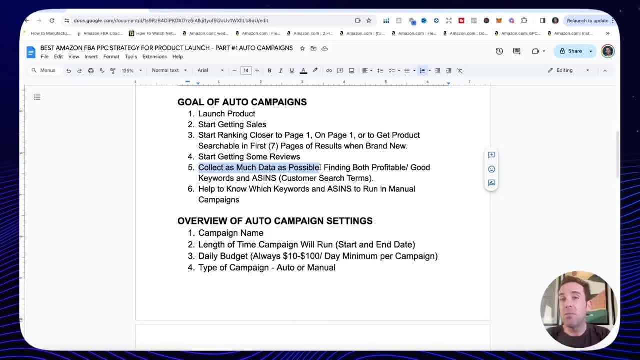 have at least a $10 to $100 daily budget. Now it doesn't mean you're going to spend eight times $10, $80 a day. It just means the campaign can go up to that. You'll have some campaigns that only spend a few dollars every couple days And you may have some campaigns that max out their 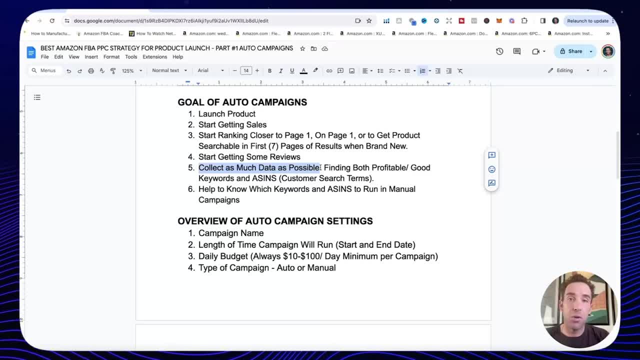 daily budget, but hopefully they're also bringing you sales And that's going to help you get more sales, And that's the whole goal. But also it's to collect data. We want to find which keywords that ASINs convert best for your product, So that way after two to four weeks you can come in and 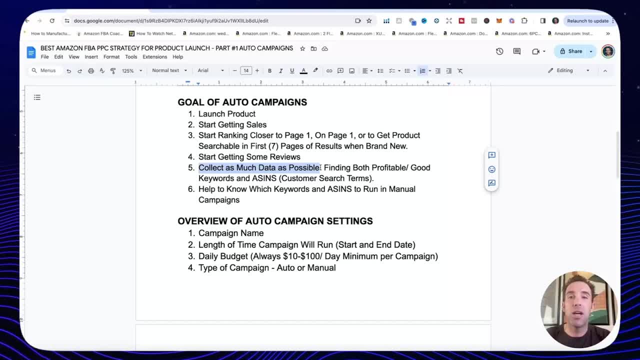 shut down some of the campaigns, just wasting money and really just kind of hyper target on the campaigns- keywords, targeting groups, ASINs- that are performing best. Okay, So we're going to be running all these different campaigns. We're going to be setting up five automatic campaigns. We're 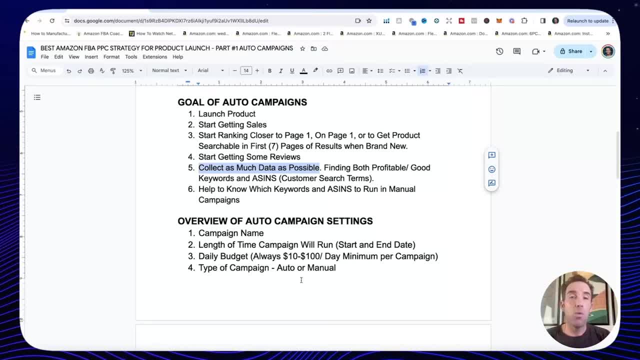 going to be setting up one or two broad match campaigns. We're going to be setting up one or two broad match campaigns. We're going to be setting up five automatic campaigns. We're going to be setting up one or two or one to three phrase match campaigns, one to two exact match campaigns. 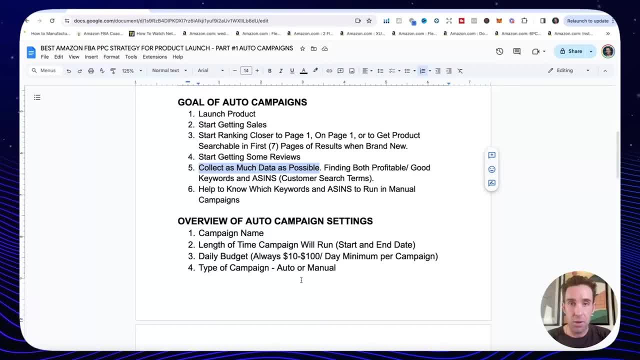 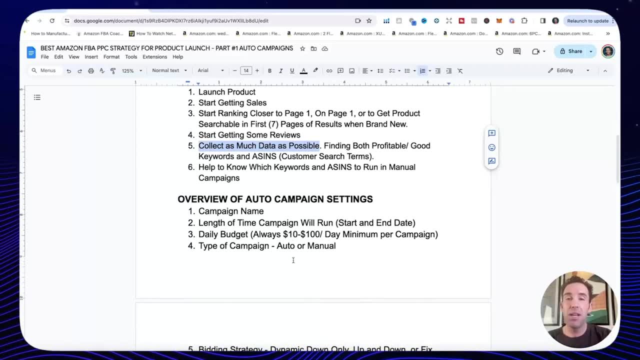 and two to five different product targeting campaigns. Okay, All right, We're going to start all those from day one. Once the listing is done, it's showing active and seller central and manage inventory And you have at least 50 to 100 units checked in. All right, So I'm going to be going. 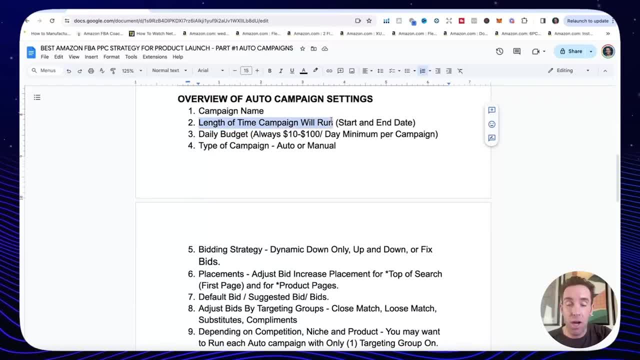 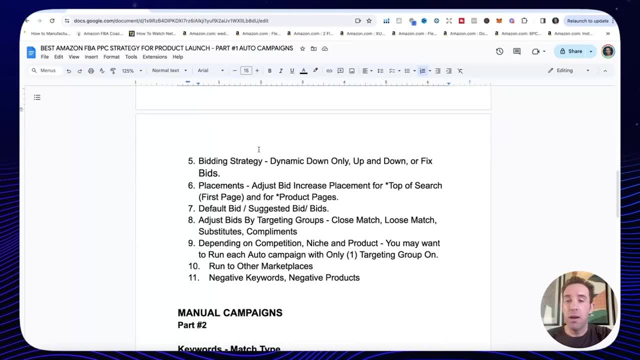 over what to name your campaign, how long the campaign should run, the daily budget you should set. what types of campaign- auto or manual- what types of campaigns you should run. what types of campaign- auto or manual- do you do? We're going to be doing both. The bidding strategy, you should. 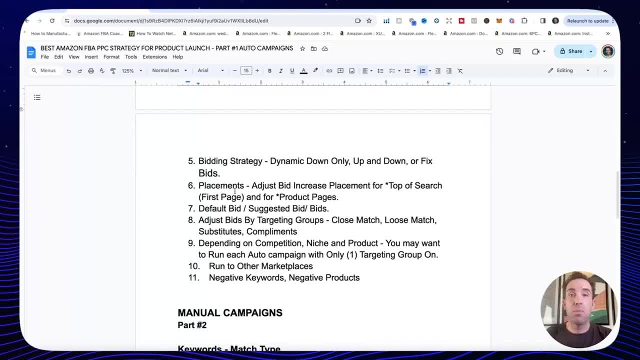 select placements. Placements are very powerful. You can use placements to get your ad shown more in the search results and get more clicks, more sales, hopefully. So definitely we're going to be wanting to use placements. How to adjust bids by targeting groups. Inside an auto you have four. 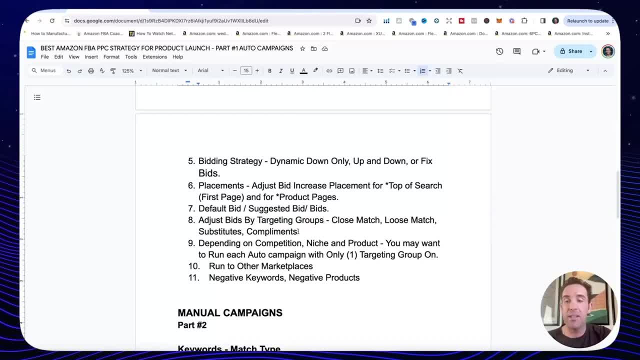 targeting groups: close match, loose match, substitutes, compliments, I'll show you that. And then do you run to other marketplaces And then how to use and when to use that And when to use negative targeting on keywords or ASINs. wasting money. shut those off. 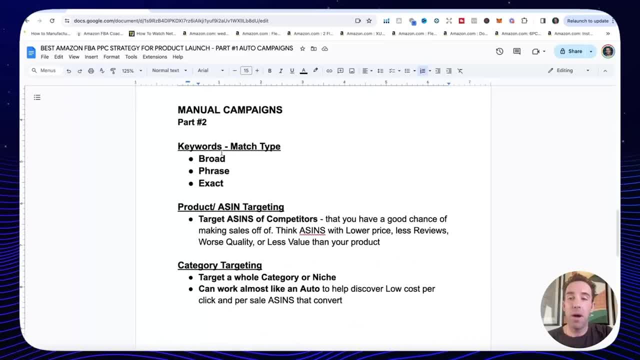 All right, And then I'll also be going over manual campaigns. The three match types for manual campaigns are broad phrase and exact. How many keywords do you put in each one? How do you segment them out based on search volume? And then how many of each type to set? 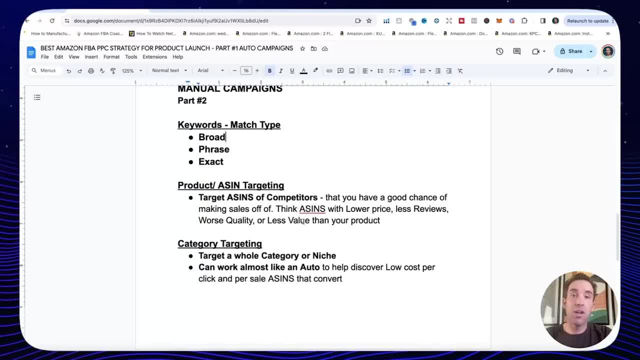 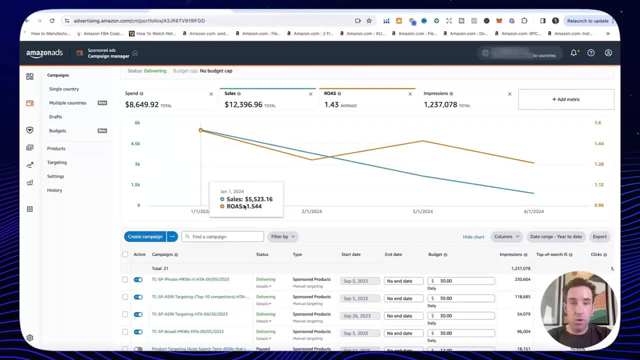 up And then we'll go over product or ASIN targeting campaigns. You want to target ASINs of competitors that you have a good chance of making sales off of? All right guys, let's go ahead and get started. So let's go ahead and start with the product and the campaign And 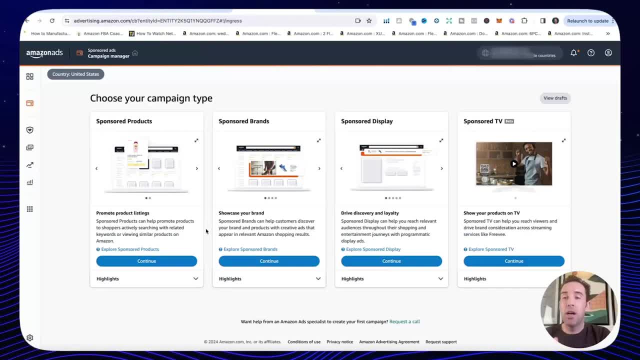 I think we're going to set up the product, So I'm going to go ahead and click create campaign. You guys can see that we have a lot of different products, So we're going to go to our advertising campaign manager. You're going to click create campaign. It's going to bring you to a screen. 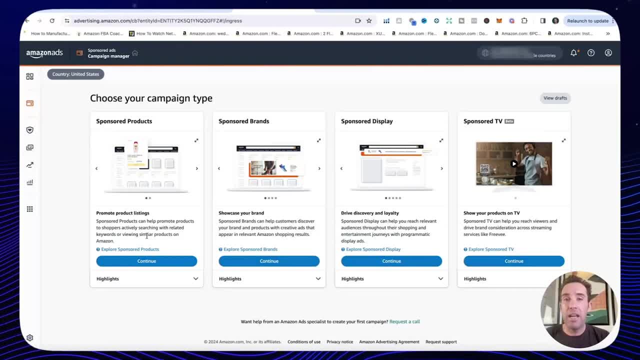 like this. Now we're going to be setting up all sponsored product campaigns. That's really all you need, guys, to launch a new product. Once you have brand registry- meaning you filed a trademark on your brand and you've submitted for brand registry and you got approval- you'll have access to these. 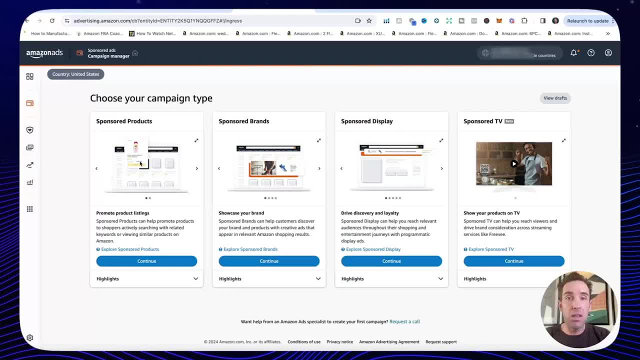 focusing on sponsored products. That's really all you need for the first month of launch And then, once you have brand registry, you've got a bunch of data from all your sponsored products campaigns. then you can slowly start going over here and running video ads, headline ads and sponsored 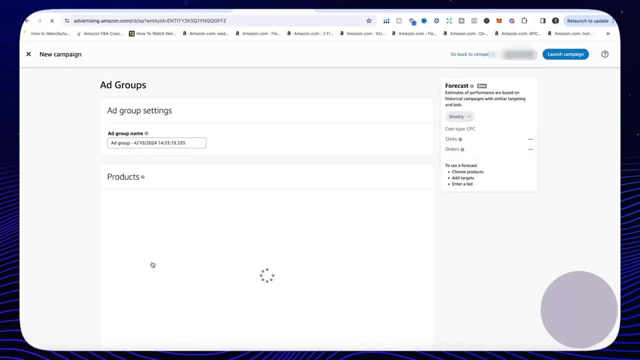 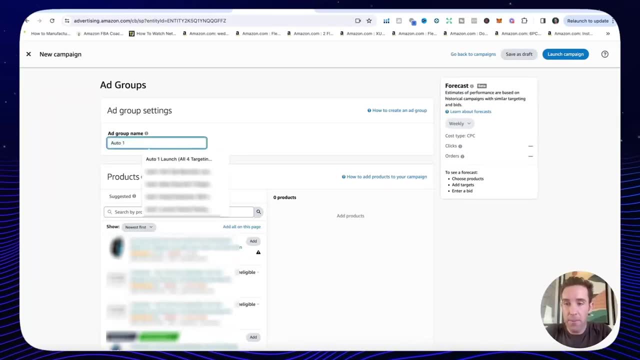 display. All right, we're gonna click continue on sponsored products. I'm going to show you first how we're going to set up these automatic campaigns, All right, So this one is going to be auto one, it's going to be ice machine, all four targeting groups. Okay, so we're putting the name. 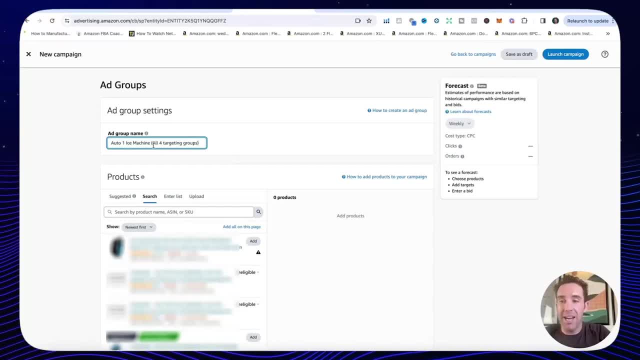 of the product We're putting: auto one, ice machine, all four targeting groups. we're going to copy this. that's going to be down below. it's going to be our campaign name. So what is the ad group? So ad group guys really don't have to worry too much about ad groups. I don't use. 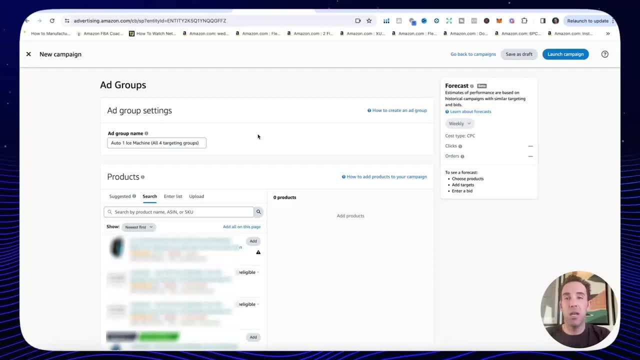 different ad groups for automatic campaigns Mostly. I'll use it sometimes in manual campaigns. It's just a different section, So I could have five or 10 keywords in ad group one and I could have five or 10 keywords in ad group two. I just recommend setting up separate. 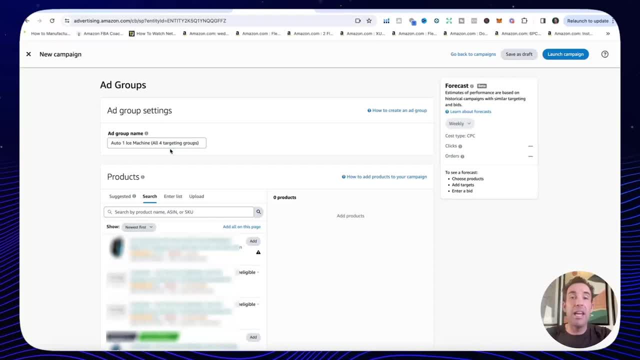 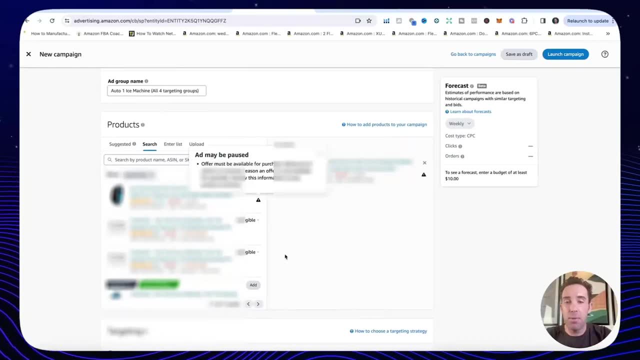 campaigns entirely, if you want to do that, But just name your ad group same as the campaign name. That's what I do. Okay, then we're going to click: add the product that you want to run PPC on. Okay, put it there, Then we're going to come down. Is this an automatic campaign or a manual? 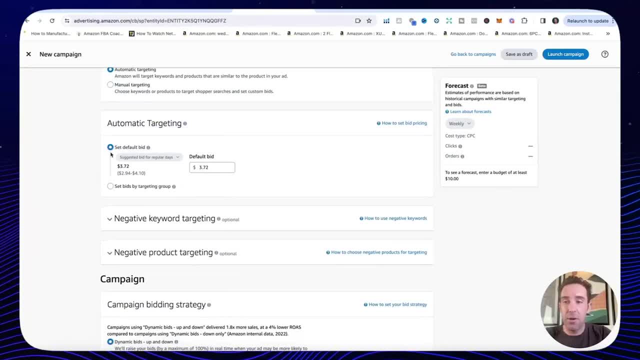 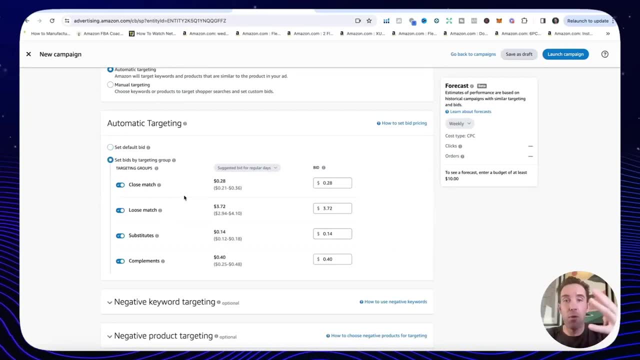 campaign. This is an automatic campaign. Is it set default bid or is it set bids by targeting group? It's going to be this one And then we're going to click: add the product that you want to run. Set bids by targeting group. Inside an automatic campaign, guys, we have four targeting. 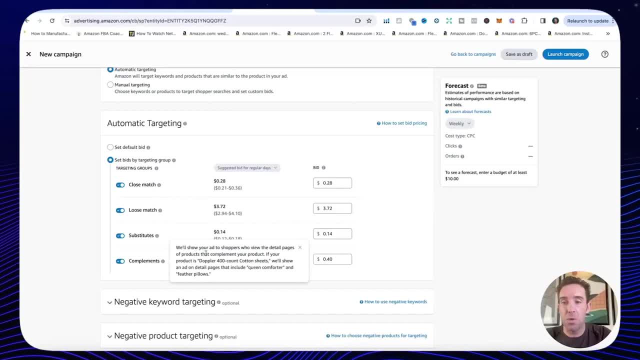 groups: Close match, loose match, substitutes and compliments. What is that? Close match and loose match are more keyword related, So Amazon's going to show you on closely related searches. So if I'm selling an ice machine for knee, Amazon may show it for a knee ice machine or a recovery. 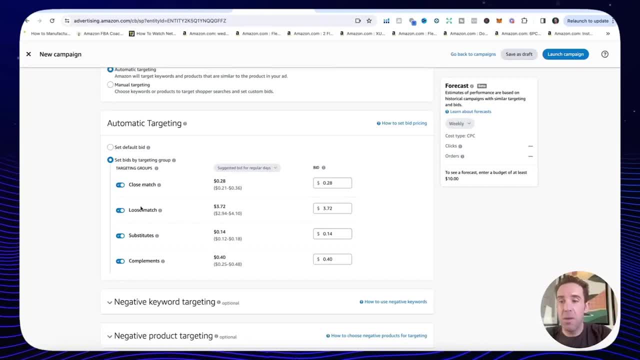 knee machine- Very closely related- Loose match. maybe the customer's not typing exactly what I'm saying, So I'm going to click add the product that you want to run PPC on, And then we're going to click add the product that you want to run PPC on, And then we're going to click add the product. 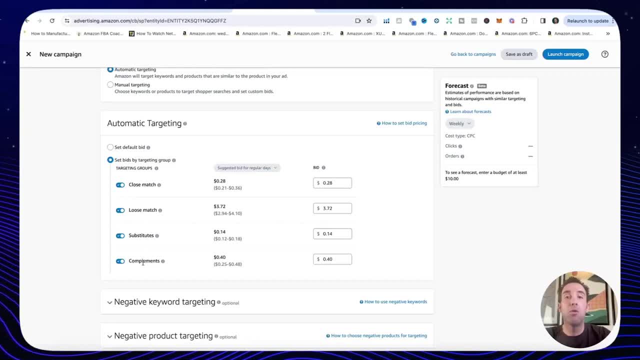 that you want to run PPC on And then we're going to click add the product that you want to run PPC on. But it's loosely related. Substitutes and compliments are going to be more product related. So switching out ASINs and showing your product over there on product pages. 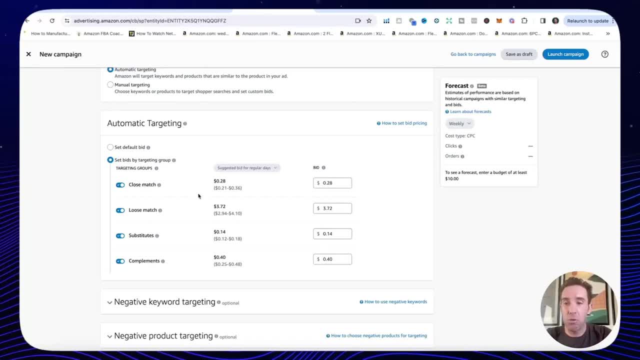 So this campaign is auto one. It's all four targeting groups turned on. Bids guys, you can increase this a little bit if you'd like. You don't have to. I usually would just go up a few cents. And the reason you don't need to go super high. you can go 10 to 20, 10 to 30 cents over the. 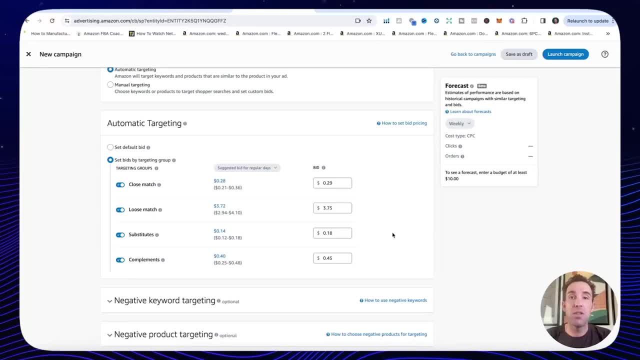 suggested bid, if you'd like. The reason I don't is I use placements to do that for me, So I'm going to show you that Next, down below placements, allow me to increase my bid, or have Amazon increase my bid instead of. 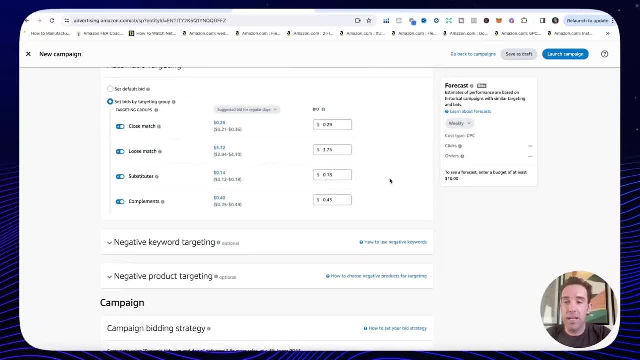 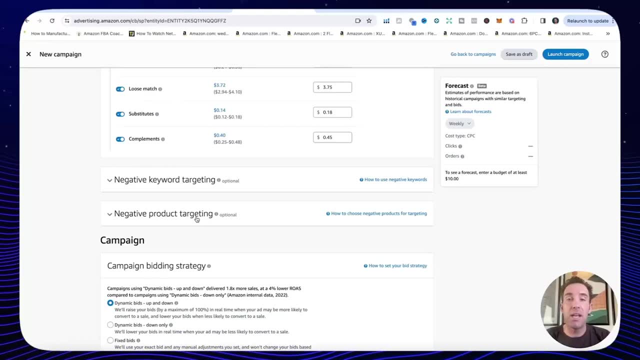 having to do it here. OK, so you can increase it a little bit if you'd like. Nothing for negative keywords, nothing for negative products. I don't have any data yet. This is a brand new product. I don't have any data that shows me which keywords or products I should negative or wasting money. 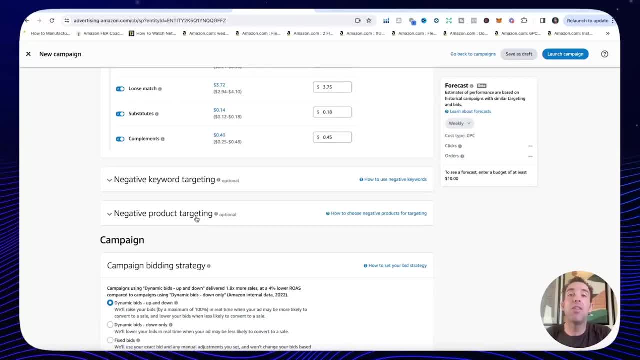 After two to four weeks you will have some data in your search term reports. Then you can negative target those ones. OK, All right, We're going to come down here. We're going to paste the ad group name, Same as the campaign. We're going to paste the ad group name. We're going to paste the ad group. 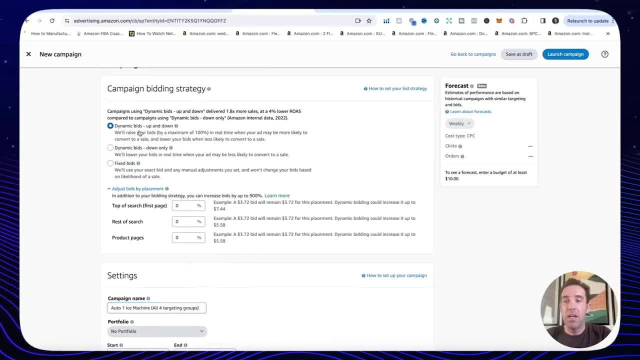 name Same as the campaign name. Let's talk about bidding strategy. All right, You have three bidding strategies: dynamic bids up and down, dynamic bids down only and fixed bids. I usually never recommend fixed bids in the beginning. You can blow through a lot of money quickly if you. 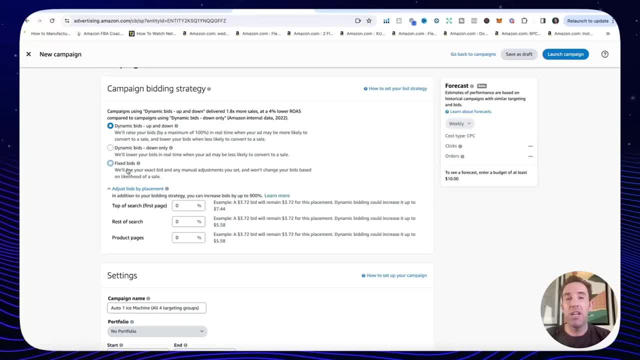 don't know what to set. You know there's no data. Even if you try to go off the data you get from Helium 10 Cerebro- suggested PPC bid or Jungle Scouts bid- suggested bid, it usually really rarely works. So we're going to be going with these two dynamic bids down, up and down. I usually 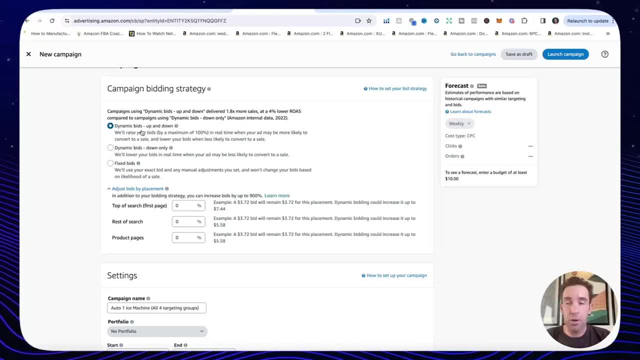 always go with that one. You're going to be safe using that one. OK, So you can do dynamic bids up and down. What does that mean? And then let me just say this: dynamic is down only. I use that one only for very specific types of campaigns. maybe for a discovery auto, a discovery category. 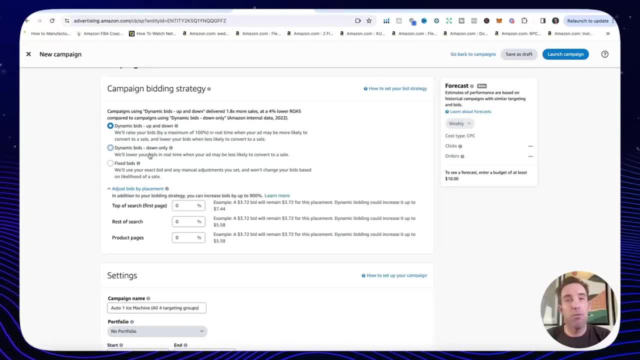 targeting campaign or like if I'm testing kind of a group of related keywords that I'm not sure are going to work, or a small group of related ASINs I would do down only to preserve the budget longer. But typically you're always going to be safe guys. 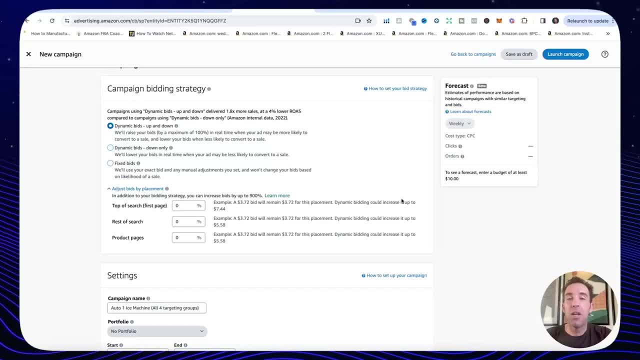 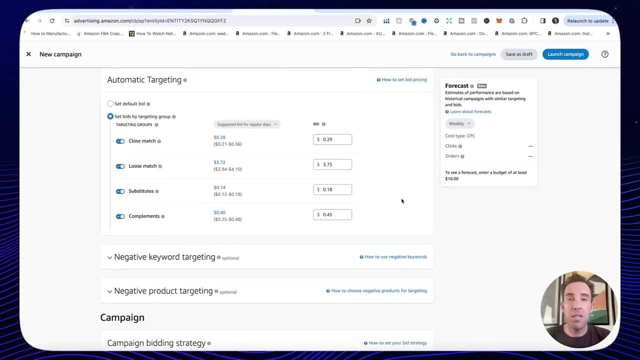 Just selecting the first one up and down. But what does that actually mean? Amazon PPC is all a bidding war. It's all about your competitors. How many other competitors are running PPC? How many other competitors are targeting the same keywords? How many other sellers there are selling your? 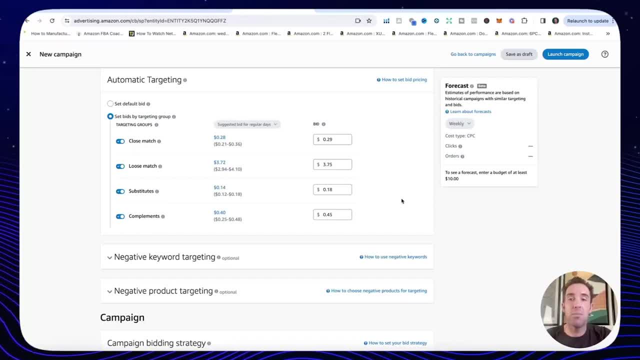 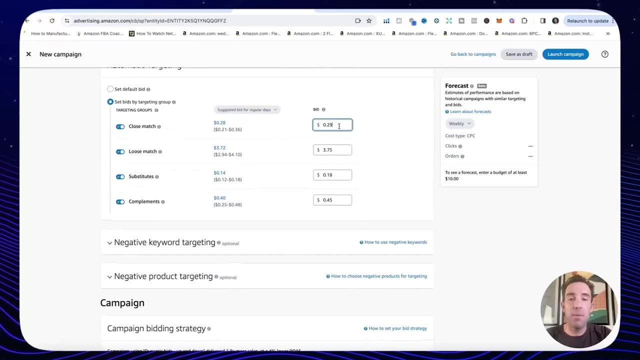 product in your category. All these things affect the suggested bid. The suggested bid does change every 24 hours, But basically how this works, guys, is you can see. I have a suggested, I have a bid set up and down. If I have this up and down selected, that means my bids at 0.29.. If my competitor is, 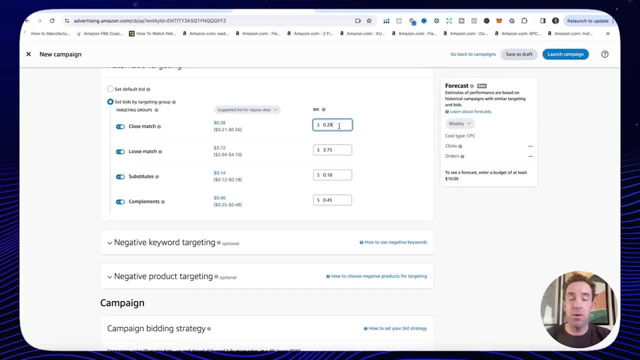 bidding 30 cents 0.30,. Amazon can increase my bid to 31, 0.31, one cent over theirs so that I would get the ad or get more placements of my ad and my listing shown to customers. If you have down only. 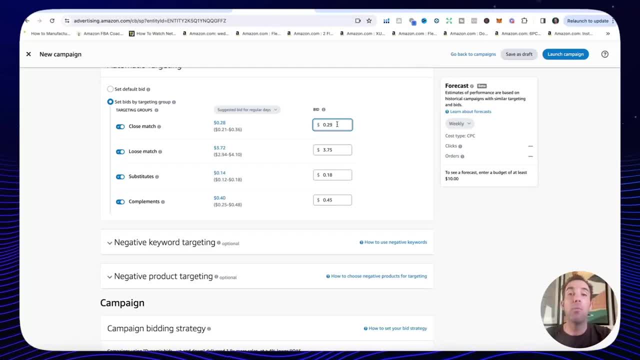 selected your bids at 0.29, the competitor bids 0.30,. you would not get the ad If you have down, because Amazon can only go down on your bid. okay, Unless you have placements going, which I'll show. 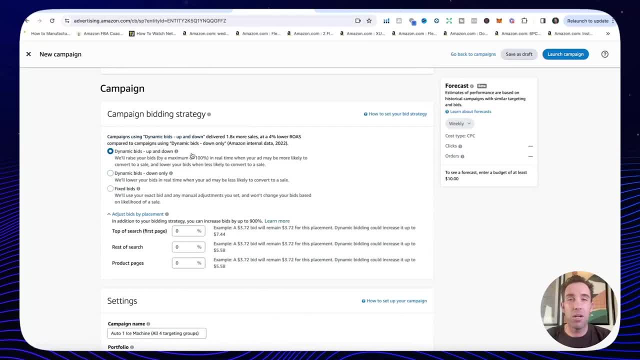 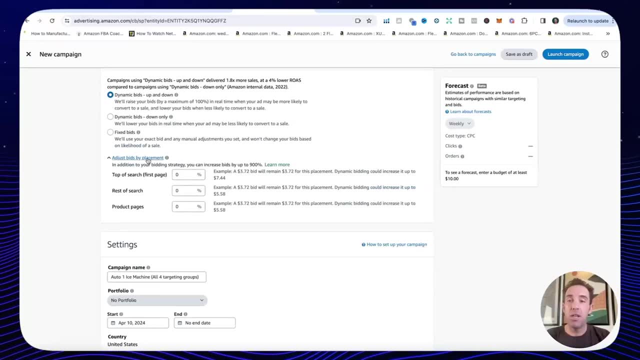 you that in a minute. So we're going to do dynamic bids up and down, basically across all these campaigns to be safe, And then here guys adjust bids by placement. Placements are very powerful because you can get more customers seeing your product and get more clicks and more sales. 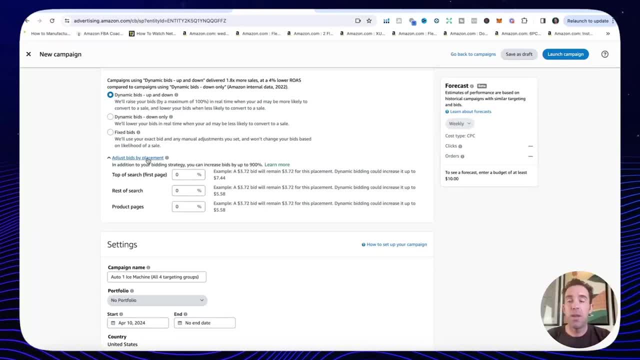 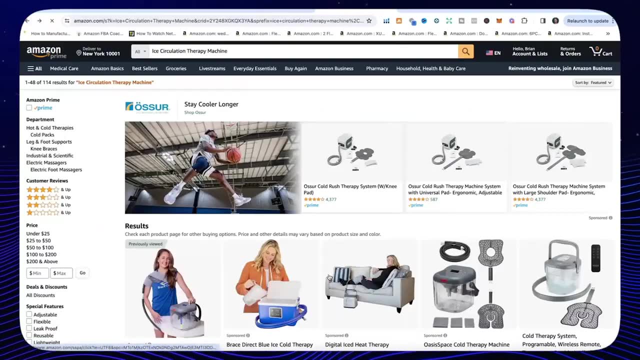 And especially during the launch phase, it's crucial to get both of those done. So what are we going to do for placements and what are they? All right guys. So when we are running Amazon PPC, there's only a couple of placements. So what are we going to do for? 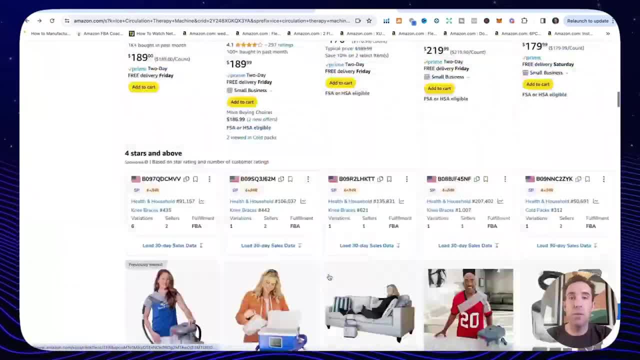 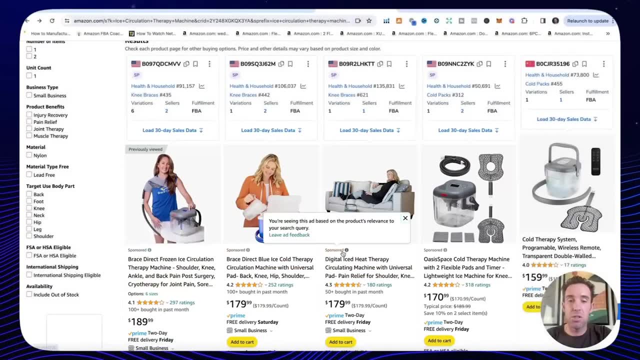 placements. We are going to run these PPC sponsored product campaigns. You can be shown at the top of the first page. that's right here You can see sponsored sponsored sponsored sponsored sponsored. position one, two, three, four. This is organic position one here. 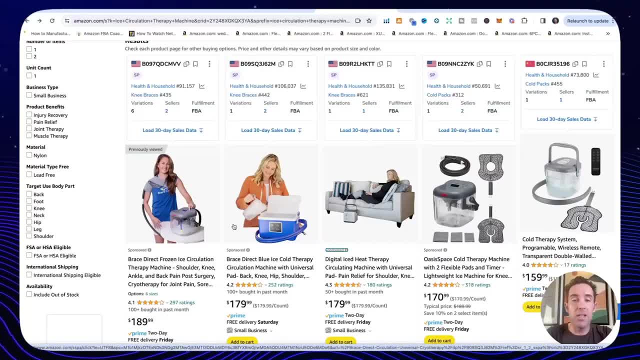 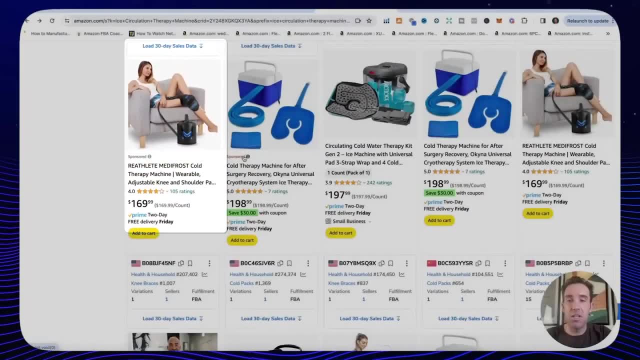 But your product may go here all right at the top of the first page. Your product may go down here, kind of in the middle of page one. There's a video ad that's different But you can see right here: this is kind of the middle of page one, That's. 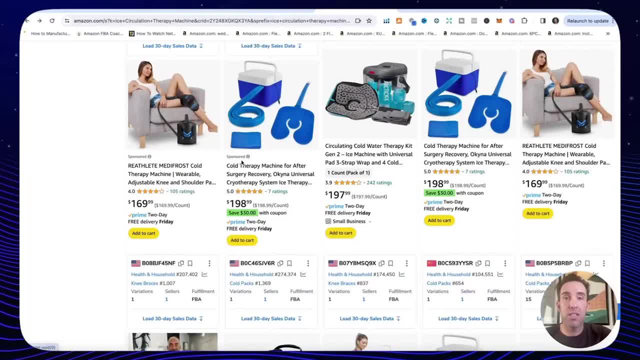 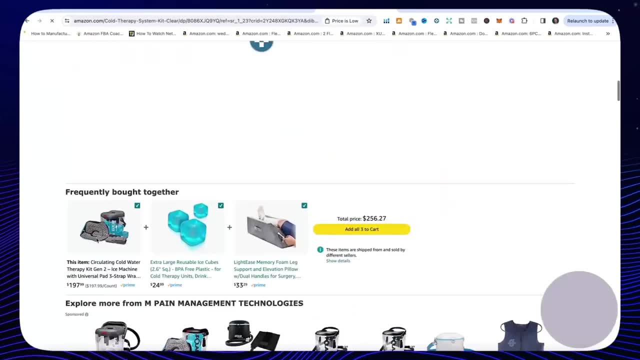 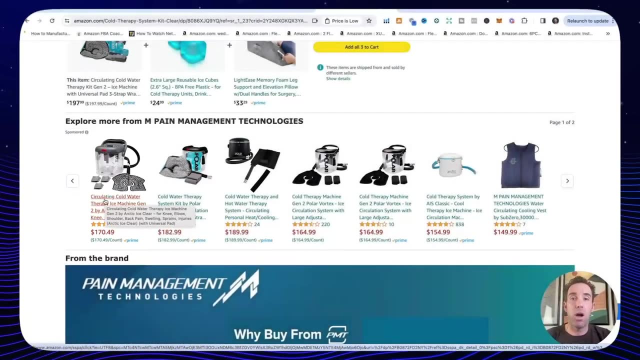 rest of search, or the top of page two. that's rest of search. or it's going to go like, right here on your competitors listing, right here sponsored. see this? uh, that's product pages. you're going to show up on your competitors listings. that's product pages, all right, and then this is a. 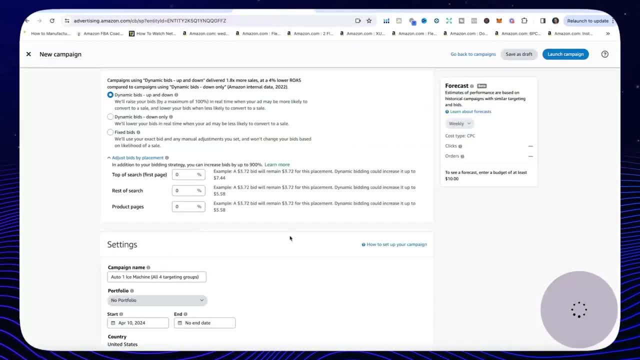 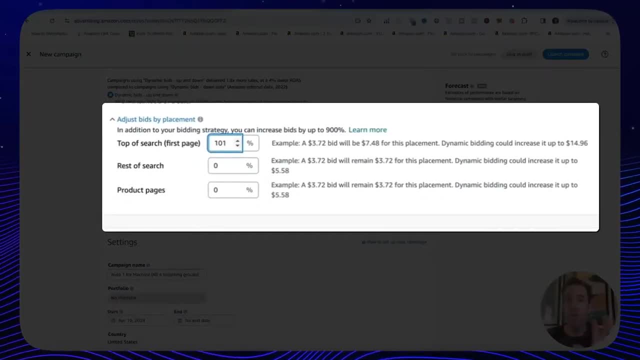 sponsored display ad right here. okay, let's go back to setting that up. so what we can do here is i can tell amazon, all right, i think my product's going to do pretty well, so i'm going to go a little aggressive on my bids. this is auto one. this is all four of those targeting groups. 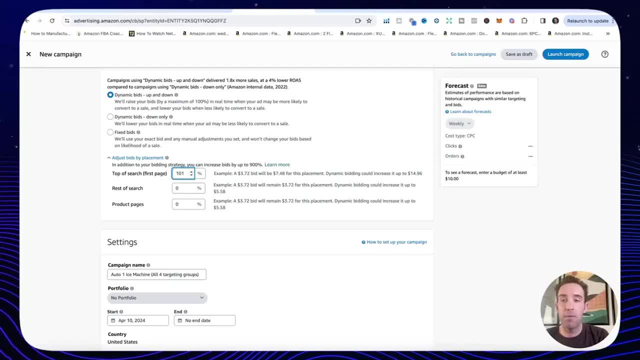 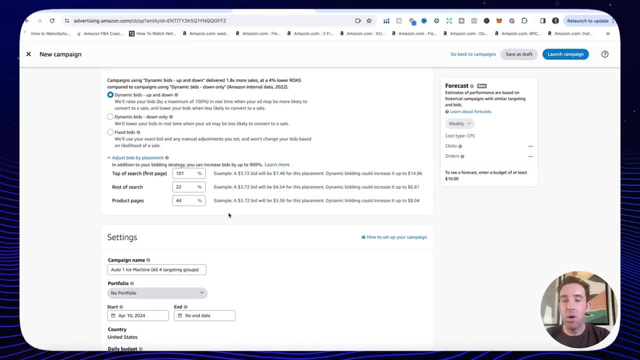 turned on. uh, i'm going to go a little more aggressive here, so i'm going to do top of search 101, rest of search, 22 product pages 44. so, uh, you just won't know what works best. typically, rest top of search will always do well for a click-through rate, because that's where amazon's 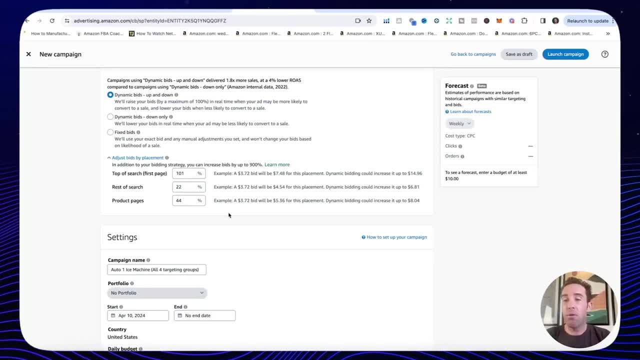 customers are going to see your product mostly, but i have some products that do extremely well on product pages. especially if you changed the product, you improved it. your offer is super compelling. your product may do really well against your competitors in product pages. that's why i like to do ascent targeting campaigns. 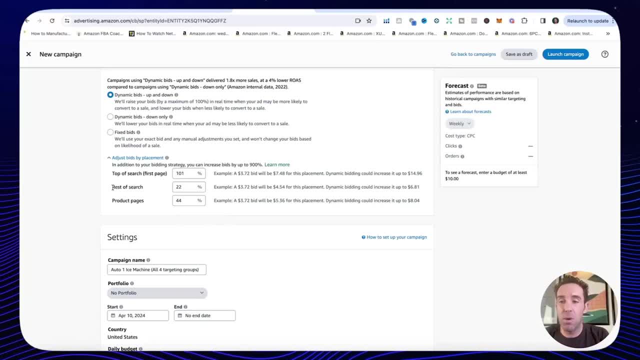 a lot of those too. or i have some products that do extremely well on rest of search. so that's top of page two, middle of page one, uh, bottom of page one, that kind of stuff. but we won't know until we run these campaigns for at least two weeks. uh, where it's performing best, all right, so we're. 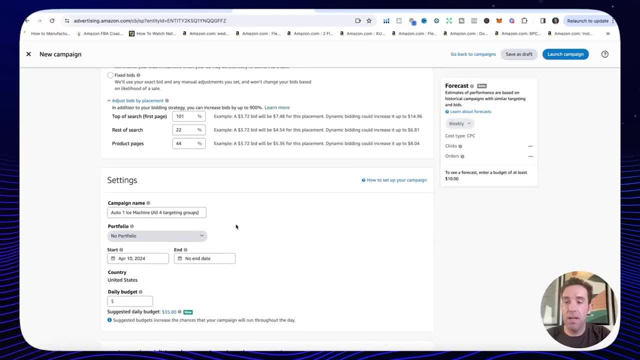 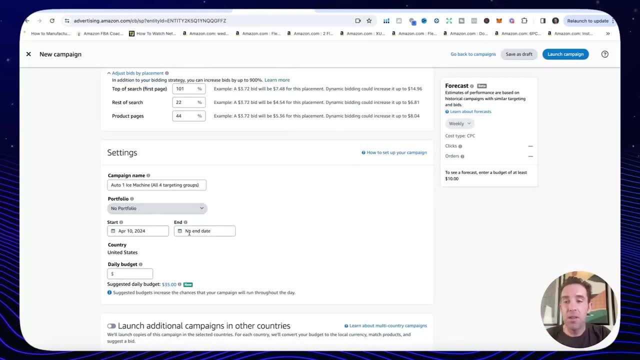 gonna set some pretty aggressive placement bids there for this auto one campaign. uh, you can add it to a portfolio or set up a portfolio. you don't have to. the campaign name same as the ad group name. this one's going to go for a minimum of four weeks. guys, i'm not going to. 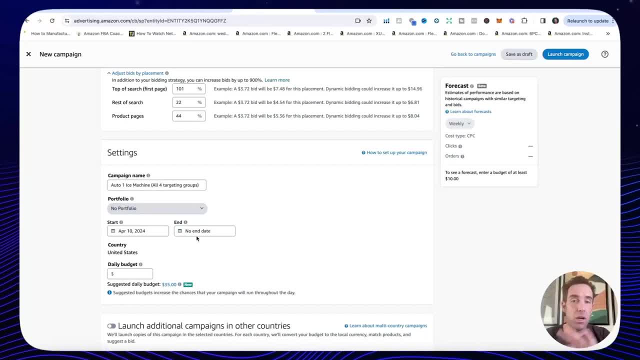 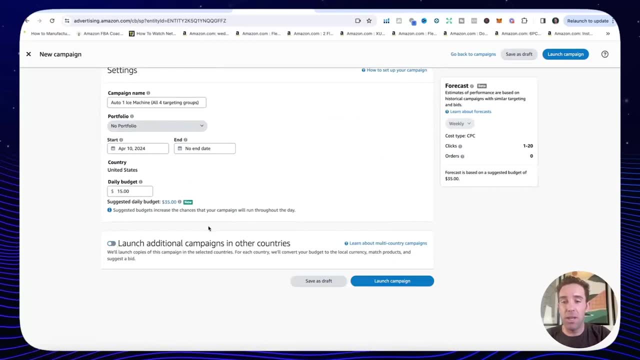 set an end date just because i always come in and check at least once or twice a week on all my campaigns. uh, the daily budget on this one's going to be 15. switch this off. we're not going to launch to other marketplaces just now and then click launch campaign and you've just successfully. 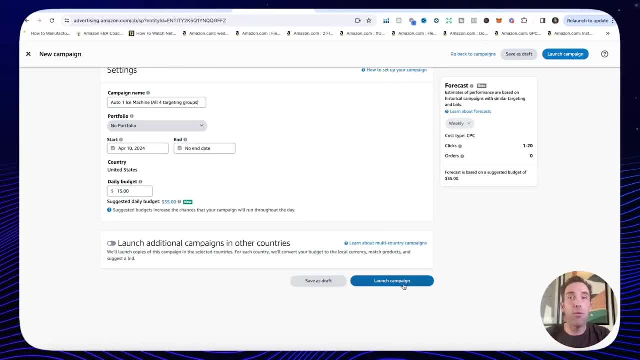 created, uh, your first automatic campaign. it's all four targeting groups turned on. that's going to start delivering right now and then you're going to set an end date for the first automatic campaign right away and hopefully getting you impressions, clicks, uh and uh, and sales- next up guys- is going to 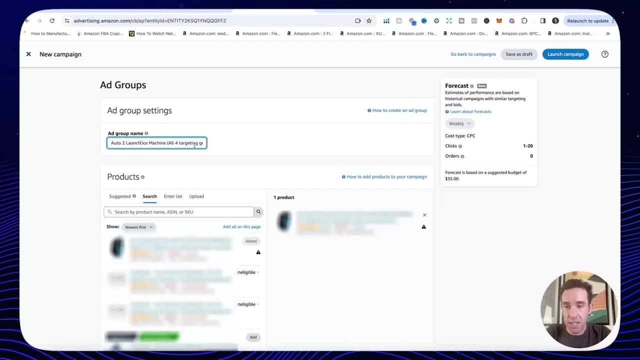 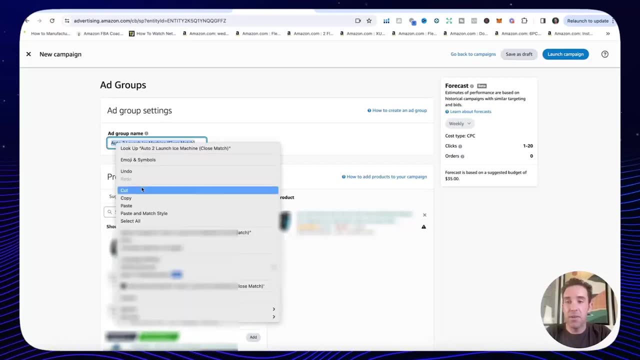 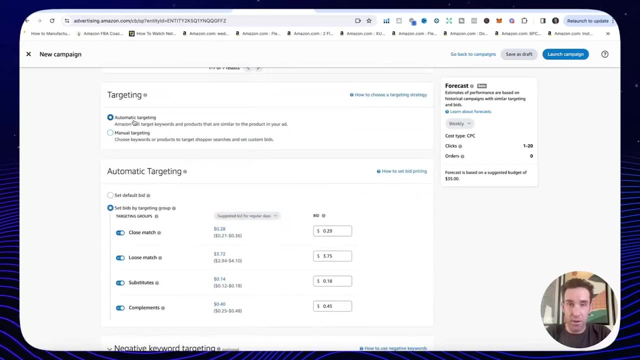 be auto two: launch ice machine. just close match. just close match. okay, we're going to copy this. we're going to add the product that we want to run ppc on. is it an automatic or a manual campaign? it's an automatic targeting campaign. next up guys here. uh, we're going to be set bids by targeting. 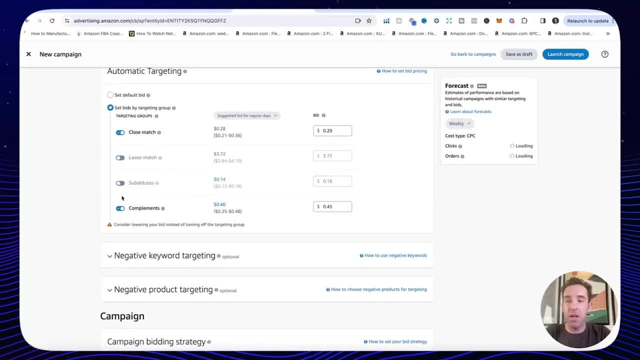 group, then we're going to switch off everything but close match. we're just going to have close match turned on. we'll increase this a little bit. okay, now why do we do just close match? and then you're going to see, the next campaign is going to be just loose match. the next campaign is going to 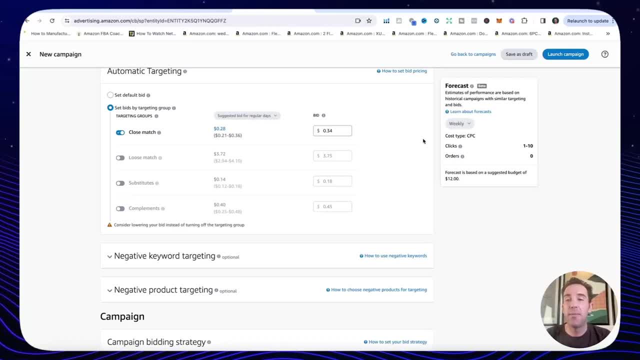 be just substitutes, and the final auto, five, the fifth auto, is going to be just compliments. the reason i like to do it this way, guys, is the auto one has all four of these on. those will typically be the bids to drive sales, uh to to start being pretty aggressive with my bidding, uh to blast my. 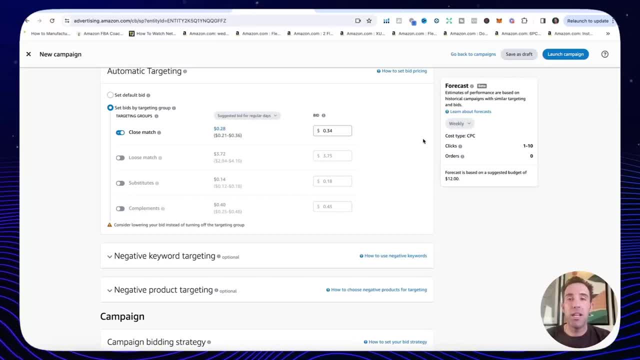 product out there, start getting reviews and all that. these ones are more to collect data. you may make some sales for them, sure, usually i will, but it's more to collect data on which keywords and asins and search terms- customer search terms- are performing best. it just helps me control my. 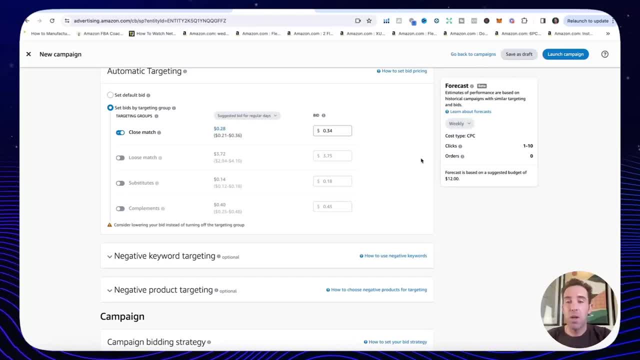 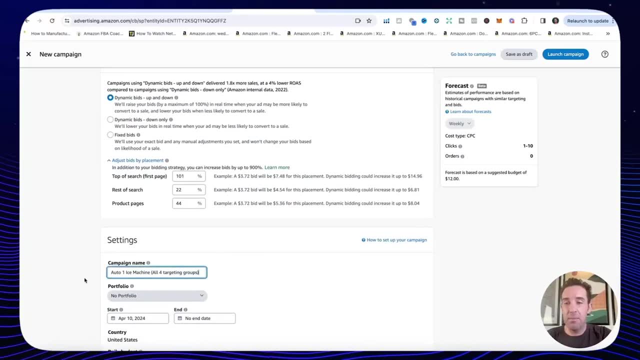 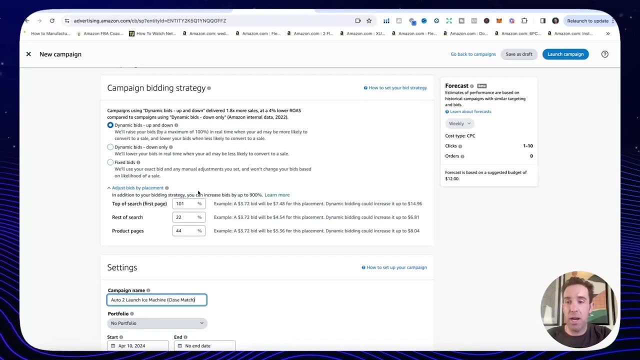 spending and amazon's spending and targeting better. all right, so we increase the bid slightly. it's just close match turned on for this auto two. we'll start with the campaign name here. auto two launch- just close match. it's going to be dynamic bids up and down again for bidding strategy. we'll be a little more conservative here on our um bidding. 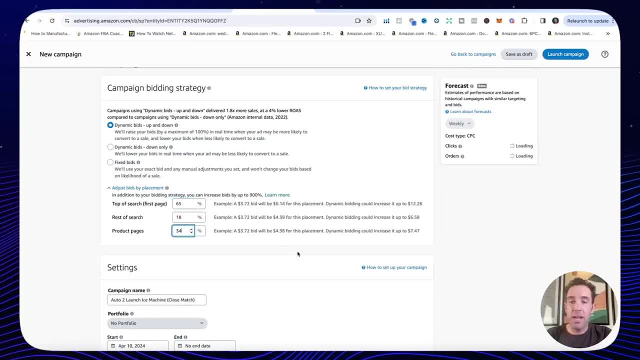 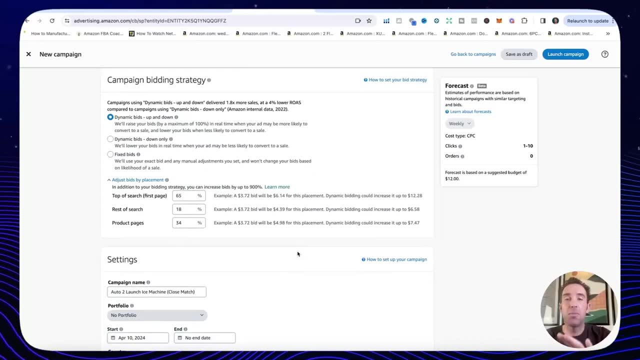 uh placement bids. okay, all right, and this is just close match. i did 65, 18, 34. you could do a little bit higher, lower if you'd like. again, we're going to do kind of these placements for at least two to four weeks and then adjust them, uh, based off the data. by the way, guys, all of the uh settings are. 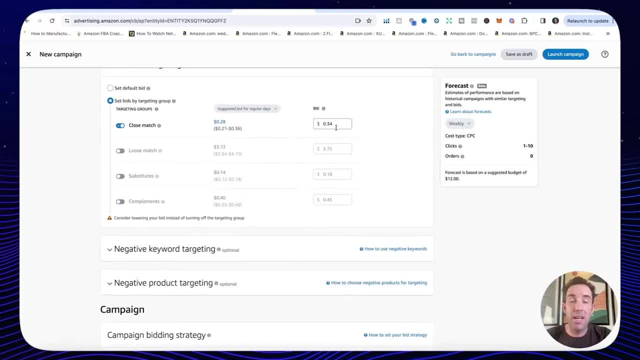 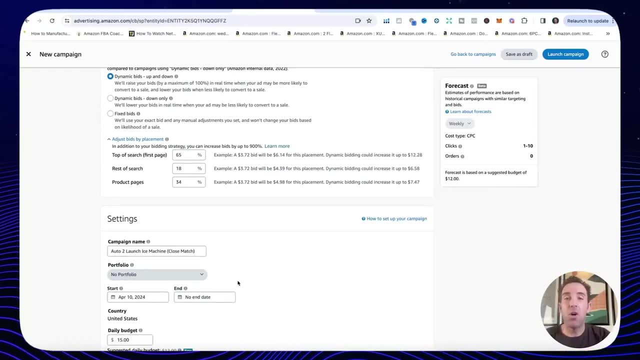 that i'm doing the campaign, um, the, the bid, the bidding strategy, the placement bids, the uh time it's going to run the budget, all of these can be changed later. in fact, after two weeks, you're going to have to come in here and change the bids, the placement bids, all of that okay, because we're 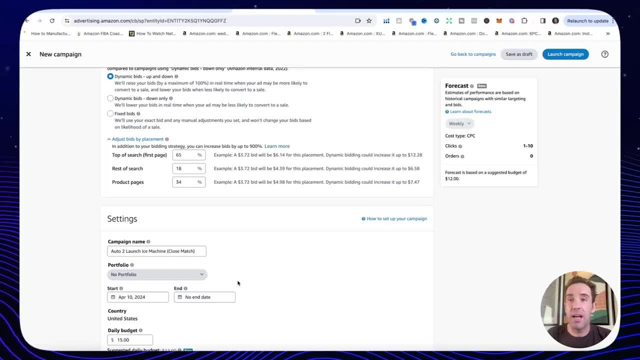 going to be looking at the data. we're going to be optimizing these campaigns at least one to two times per week based off what's working and what's not working. we're actually going to be shutting down the bids that don't work so that you can really just start focusing on what's driving the. 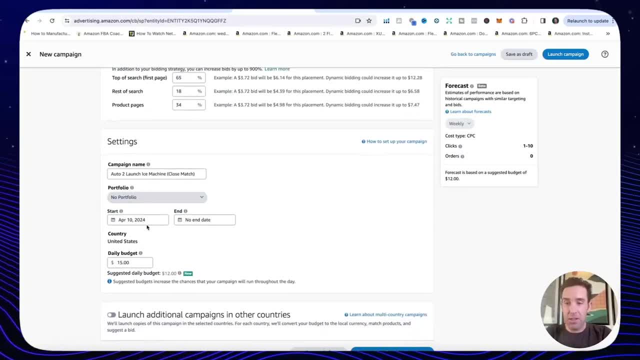 most sales that kind of stuff. okay, all right. so we've set the campaign name. it's going to run for at least four weeks- i'm not going to set an end date because i can just shut it off- and then it's going to be a 10 daily budget on this auto 2 and then launch campaign. all right, now we've just set. 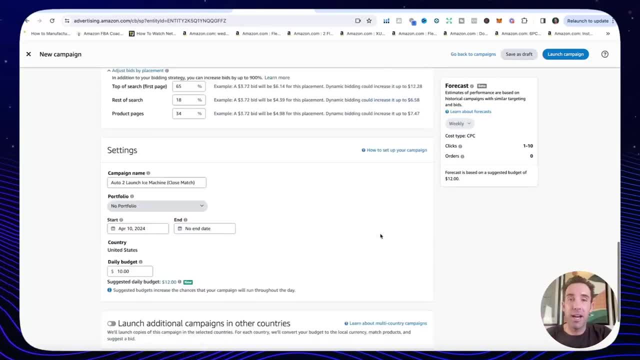 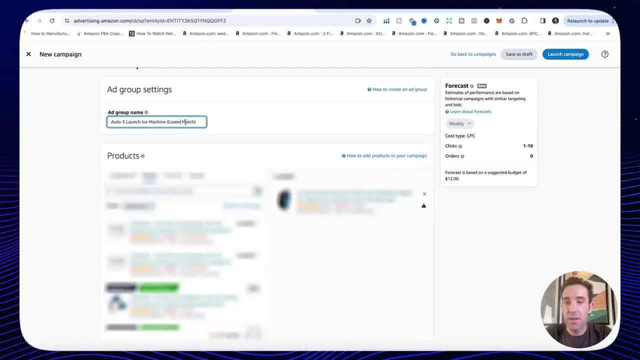 up an auto one and auto two. you're going to do three more autos, guys, just like i just walked you through. it's going to be auto three. it's going to be loose match only. okay, we're going to add the product. it's automatic targeting. this one's just loose match, turned on. 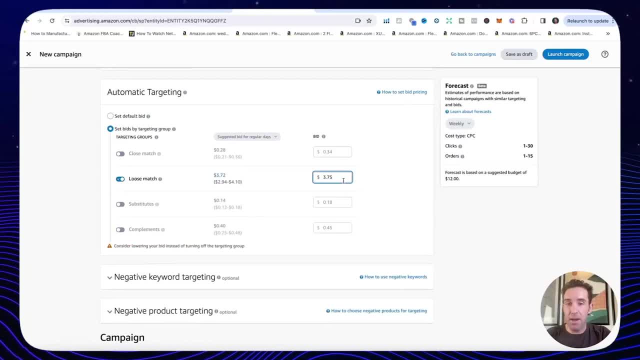 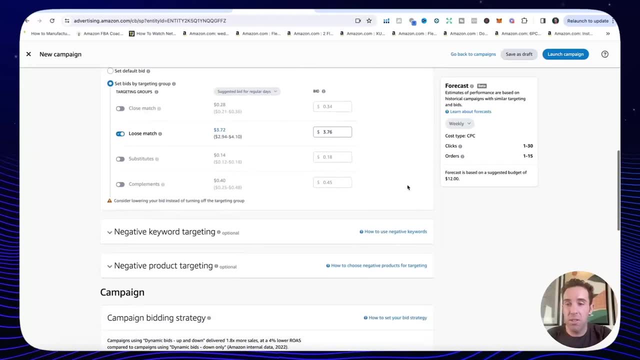 everything else switched off. that's a really high bid. um, i'm not sure where that's coming from, but i'm not going to go much higher than that. that's super high. again, these suggested bids will change every 24 hours. nothing for negative keywords, negative products. we're going to do dynamic. 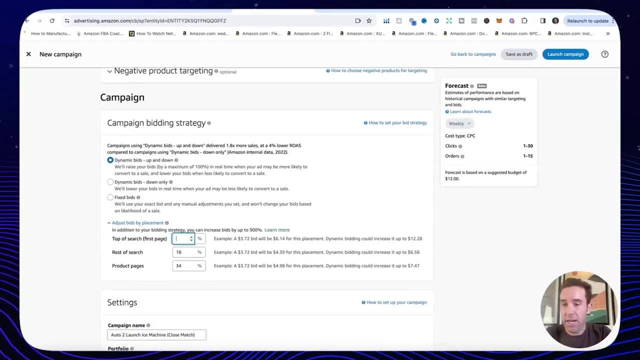 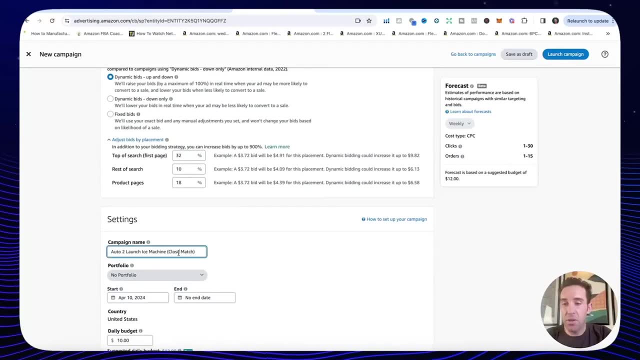 bits up and down. uh, that bit is already really high, so i am going to bring this down. okay, if that makes sense, why i'm doing that? this is just loose match. uh, then this will be just loose match here for, uh, auto three, all right, and then again same thing. 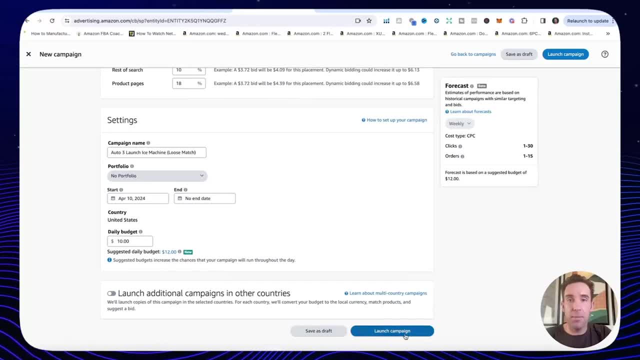 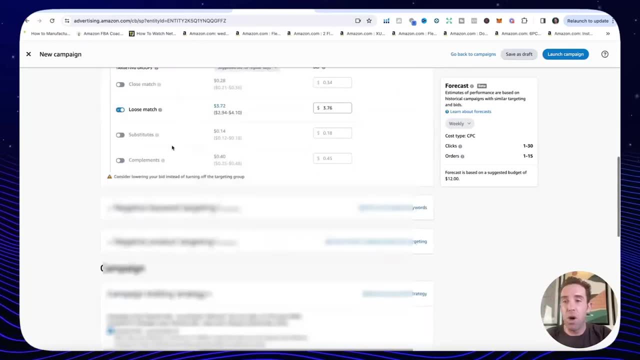 it's going to run for four weeks. it's going to be a ten dollar daily budget and launch campaign. all right, guys. so now we've just set up three. walked you through setting up three autos. you'll just set up two more. you're going to set up one, uh, one more auto for just substitutes. turned on all the same. 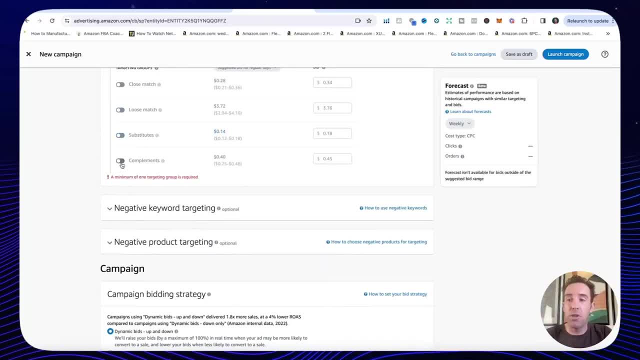 settings below and then come back in and set up one more auto for just compliments turned on, all right. so we're setting up all your automatic campaigns. now let's go over setting up your manual keyword targeting campaigns. so manual keyword targeting campaigns. let's go over that. 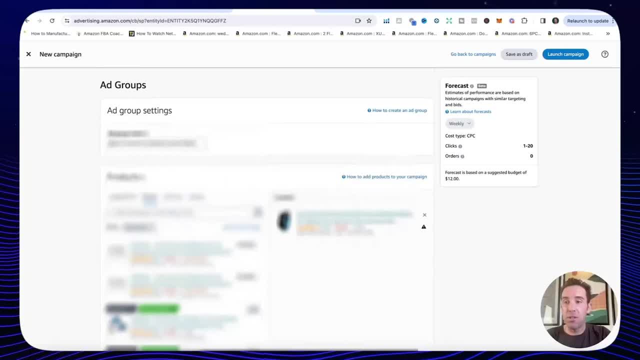 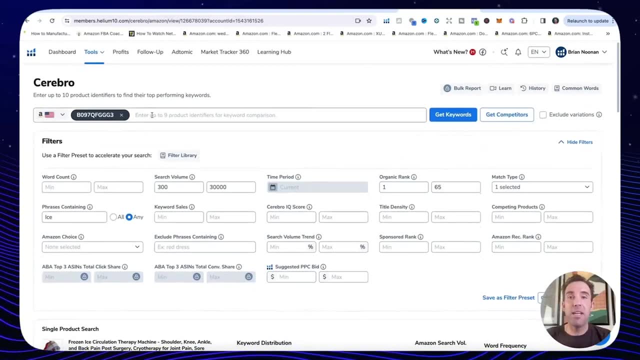 uh, all right. so, first of all, where do you get the keywords that we're going to be running? all right, you're going to come to Cerebro from helium 10.. you're going to paste the top five to ten competitors asins in here. click on get keywords. you're going to do some filters- 300 to, let's say. 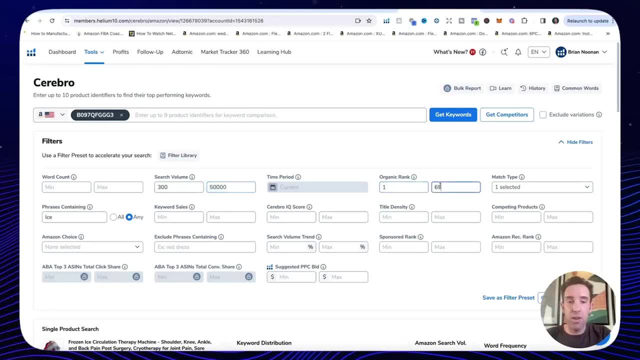 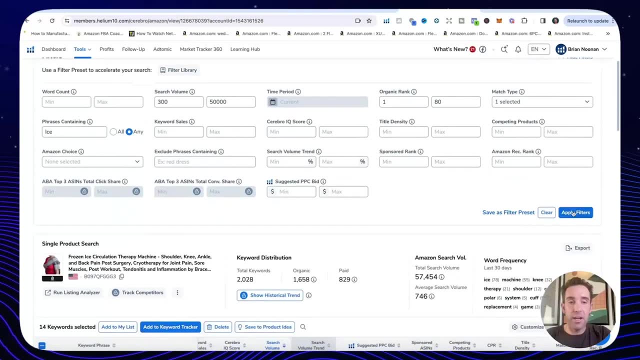 50 000.. organic rank one through, let's say, 80.. that's page one. two, three roughly match type is going to be organic and then click on apply filters. how many are we left with? we're left with 82 keywords. that's very manageable, so. 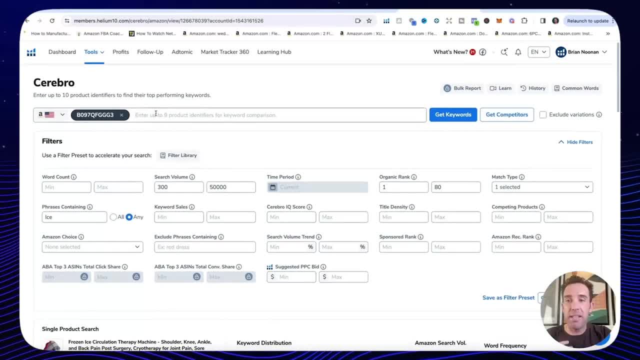 did that make sense? how I did that? I did five to ten of my competitors. asins here pasted that. uh, I did 300 to 50 000. search volume: filter organic, rank one through 60 or one through 80, match type: organic. and now I'm left with kind of the best keywords for this product. 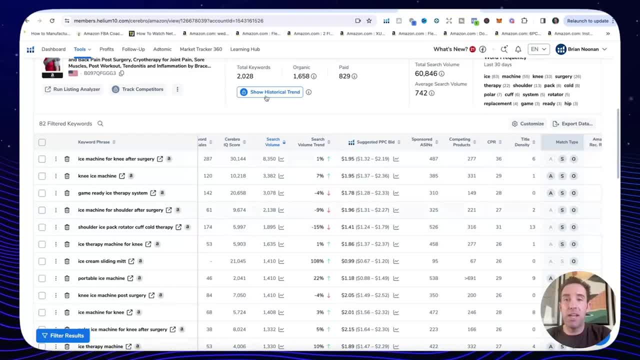 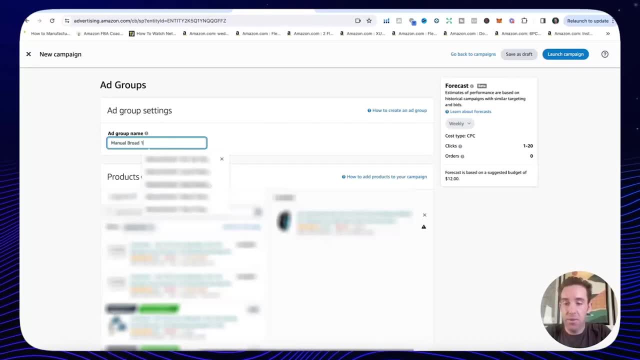 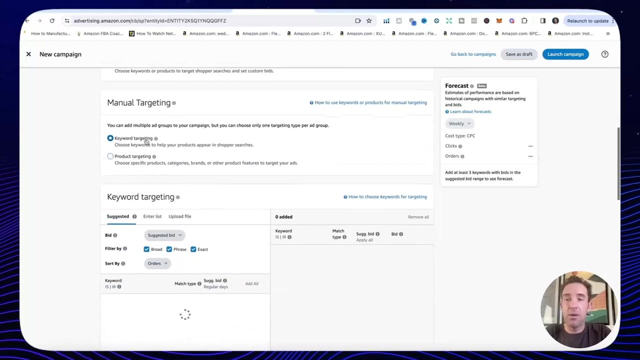 all right. so how do you go through here? well, uh, what we want to do is we're going to be setting up a campaign. this is going to be manual, broad one, top 10 keywords. okay, we're going to add the product and it's a manual targeting campaign. is it keywords or product targeting? it's keyword targeting next. 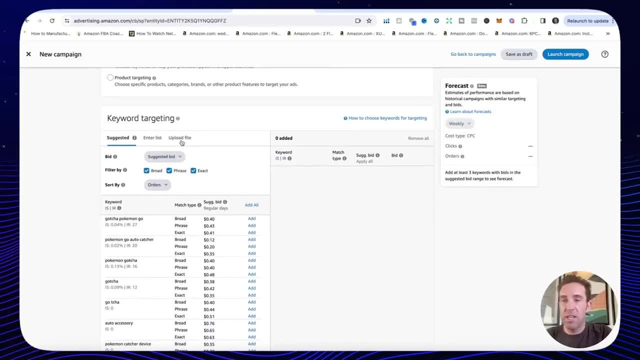 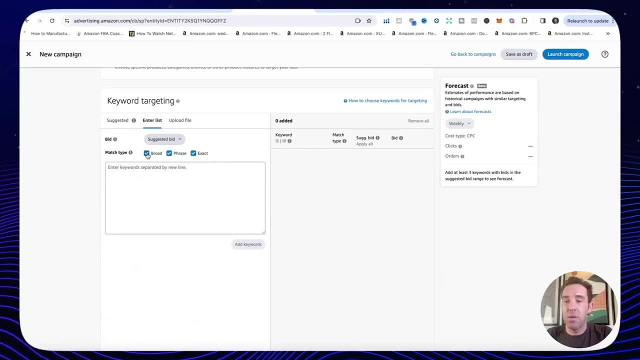 up. are we going to do suggested keywords? uh. interlist upload file. you can look at some of the suggested keywords if you'd like, but we're going to be entering a list. uh, it's going to be just broad match, all right now. here's where it. 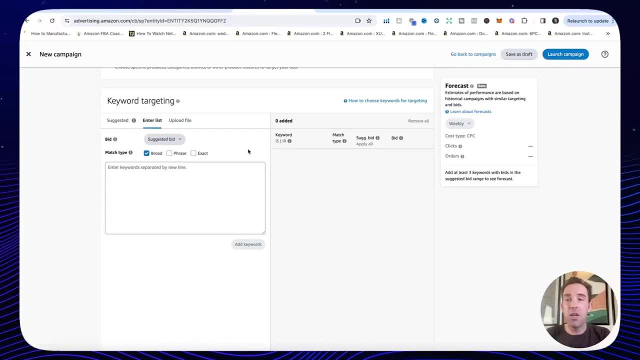 gets uh tricky when you set up these manual broad campaigns and phrase campaigns and exact match campaigns. you have to segment them out. so we're going to be setting up just broad match campaigns with roughly 5 to 15 keywords in each broad campaign. then phrase is going to be a whole. 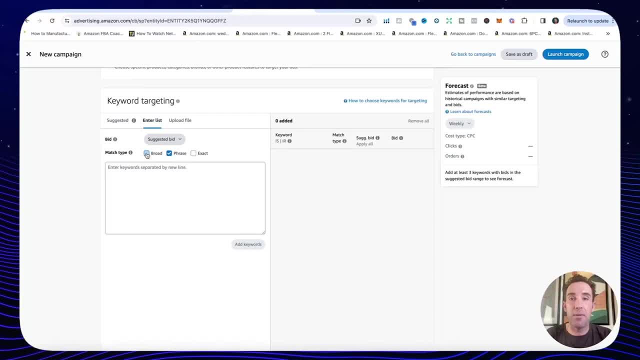 other campaign just phrase match in that camp. those can't those keywords just phrase match in their own campaign and then you're going to set up an entirely different campaign just for exact match. so we're creating different campaigns with 5 to 15 keywords in each for just broad match and just phrase match. okay, for exact match. I only do one to three keywords per exact match campaign, and not only do we want to separate them out based on match type, you also don't want to put a keyword like this one ice machine knee for knee after surgery, with 8 300 search volume. you 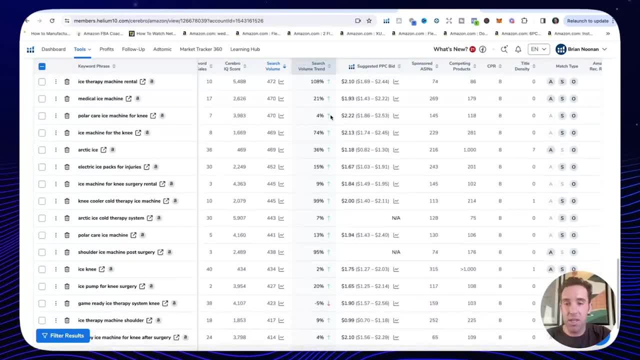 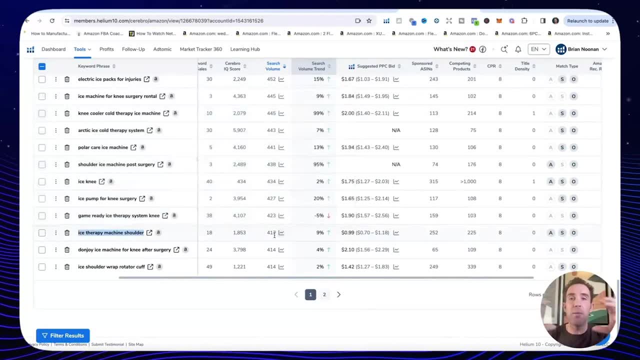 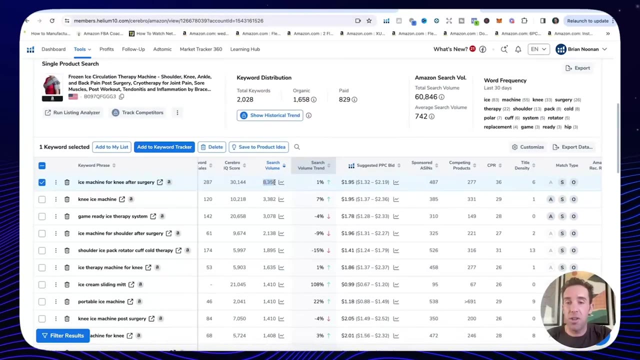 wouldn't want to put this keyword in this campaign. with this keyword down here, ice therapy machine shoulder- it's only got 400 search volume. if you end up putting those two keywords in the same campaign, it's not going to work. Amazon is going to spend all your money, your budget, on this keyword. 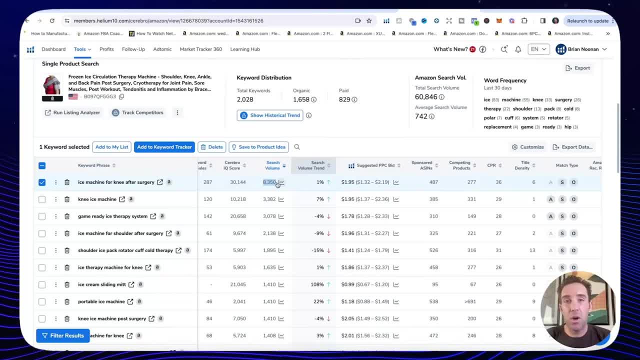 with the high search volume and you won't get any much data on the lower search volume. so you're not going to get a search volume keyword, even though that lower one may really work. so we're going to set up different campaigns based on the match type. broad has their own, campaign phrase has their own. 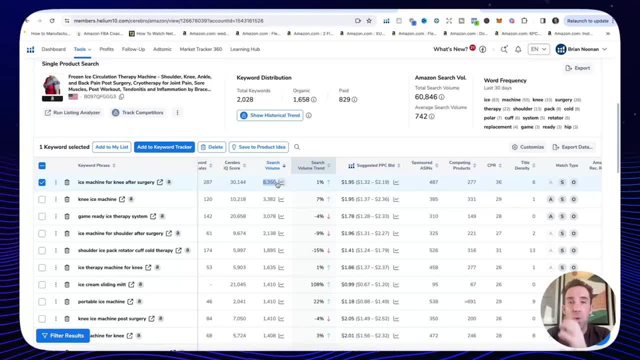 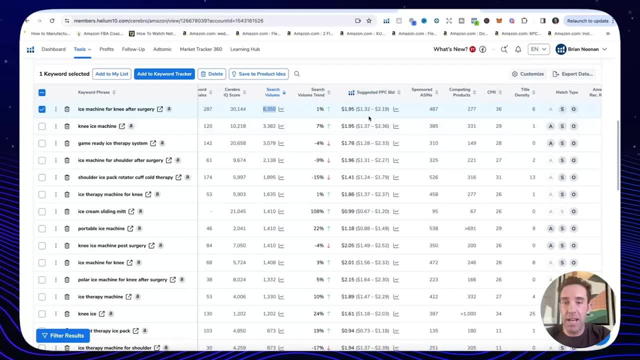 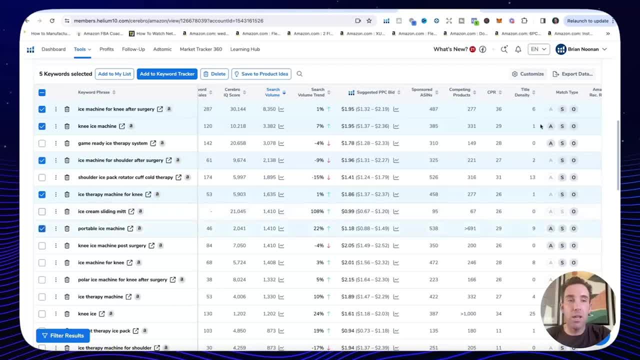 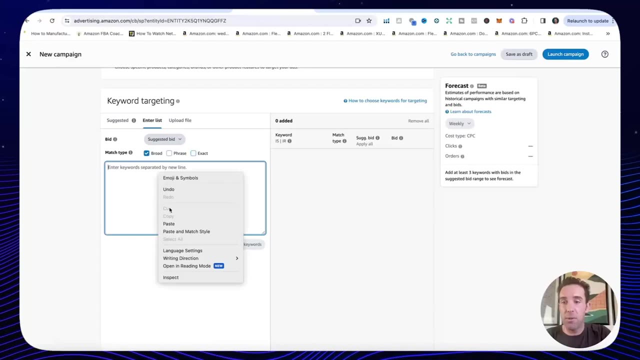 let's say those uh five. okay, I would click on uh export to CSV file or to Frankenstein to process the keywords quickly instead of copying them one by one. but then we're going to copy the keyword, we're going to go over here, we're going to put it in here. this is just broad match. we're going to paste it here, click. 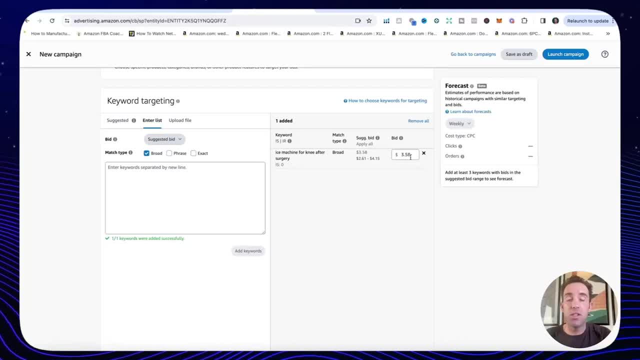 add keyword, it'll move it to the right. I would just go with the suggested bid for now, and then you're going to do that with these other ones and I'm just going to do these five keywords, because these are higher search volume keywords. um, I would just do it like that. so add the other three. you're going to have roughly five to ten. 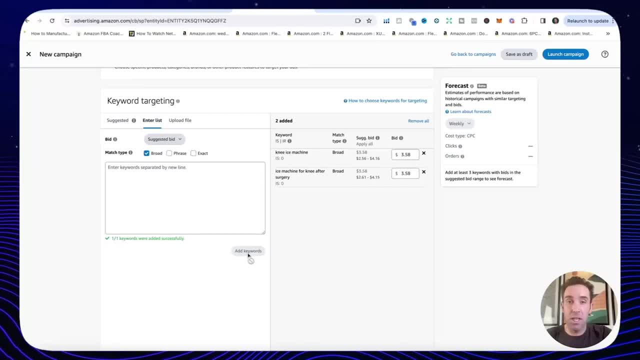 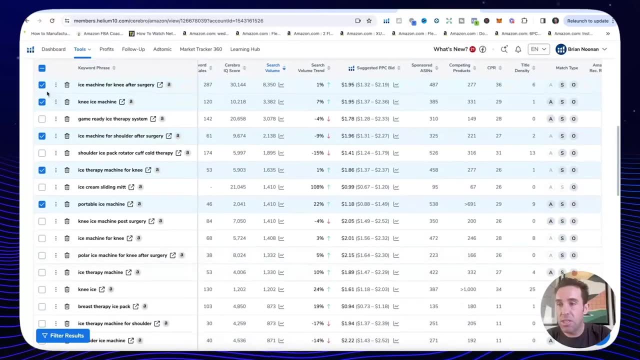 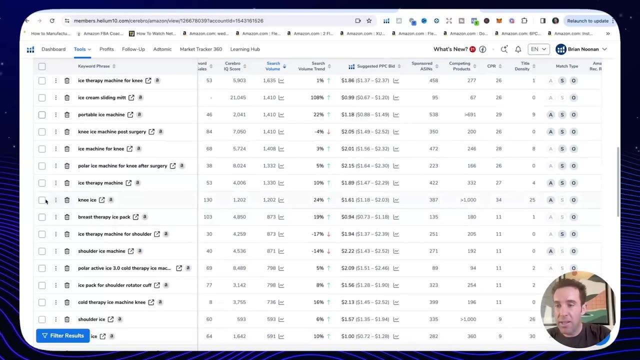 keywords in this broad one and then I'll finish setting this campaign up and then I'd come back in and set up another broad campaign, broad two, with like 10 keywords down here with lower search volume, so probably like 1 000 or under. so I would go like this one and this one and this one and 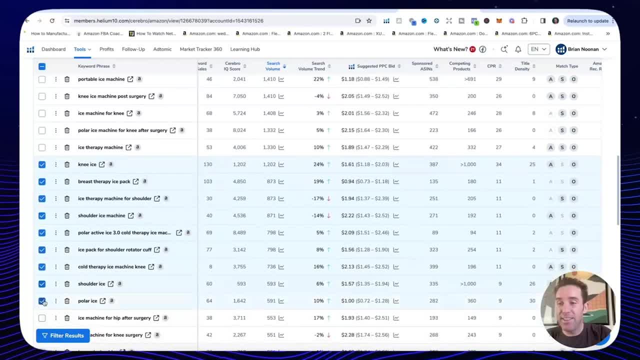 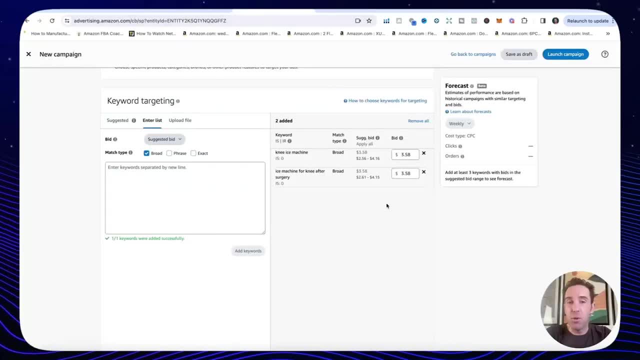 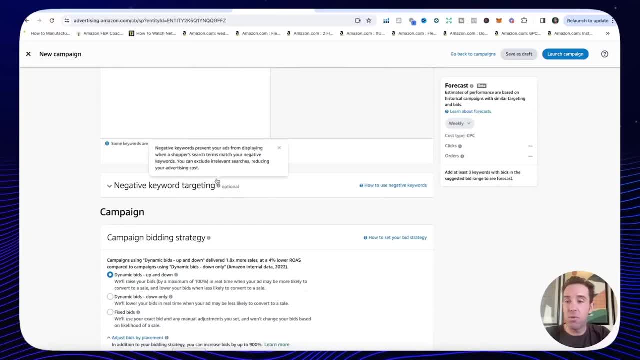 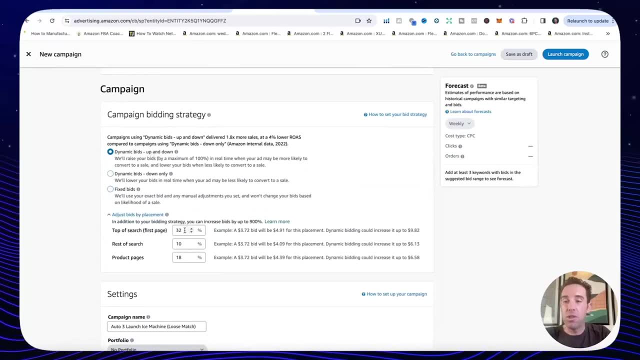 match and just leave it at the suggested nothing for negative keywords. we don't have any data yet that tells me which keywords are too expensive. it's going to be dynamic bids up and down. we're going to use some placements. we don't have to be so aggressive here with placements, but I do like. 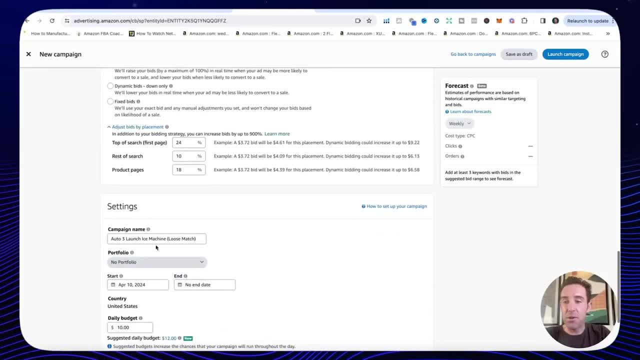 to set some. okay, we'll set it like that. it's going to be manual broad one, it's actually like top five keywords instead of ten, but you can bring it round one, launch something like that, so you know okay, and then it's going to run for at least four weeks. two, 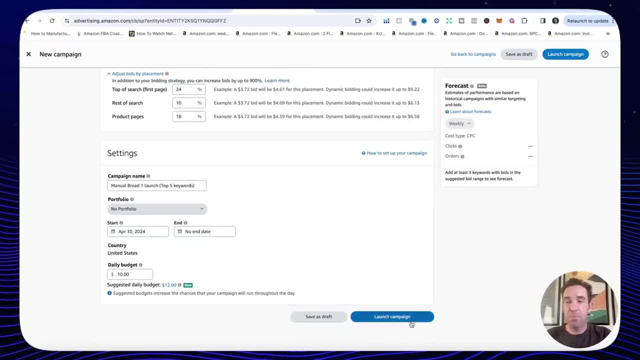 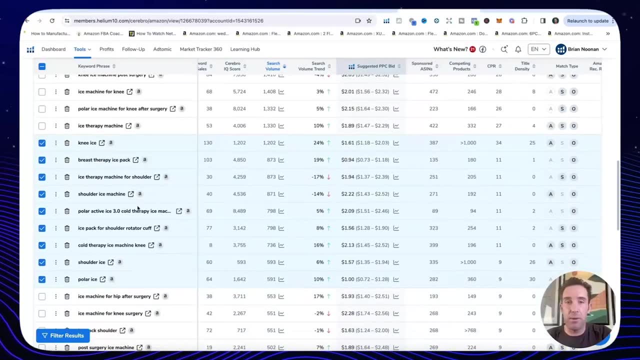 to four weeks. it's going to be a ten dollar daily budget, then click launch campaign. so I've just set up broad one. then you want to come back in and do broad two, same settings with these 10 keywords down here. then for phrase you're going to do the same thing, except for when you come over here. 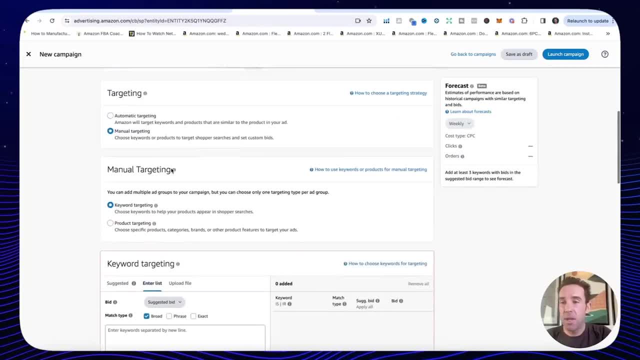 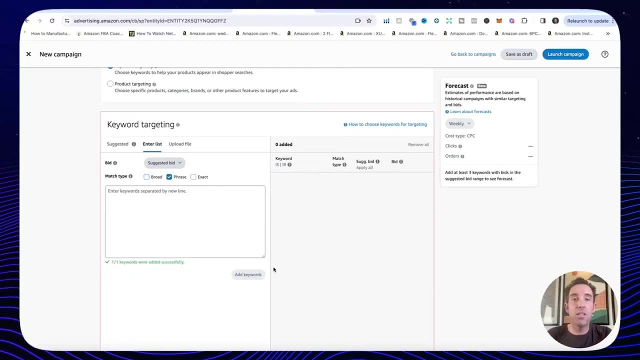 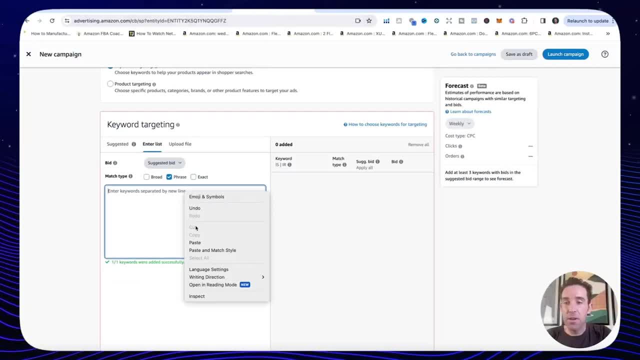 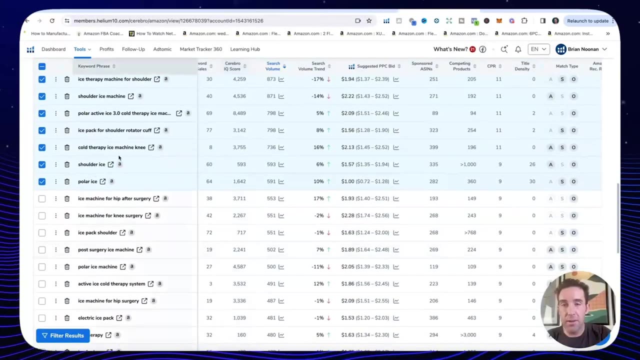 this keyword, copy and paste it into here, okay, and just phrase match, do those five keywords, and then we're going to launch that one and we have phrase going okay, with those five keywords. then we're going to do another phrase campaign with these keywords down here. okay, 10 of those, so no more. 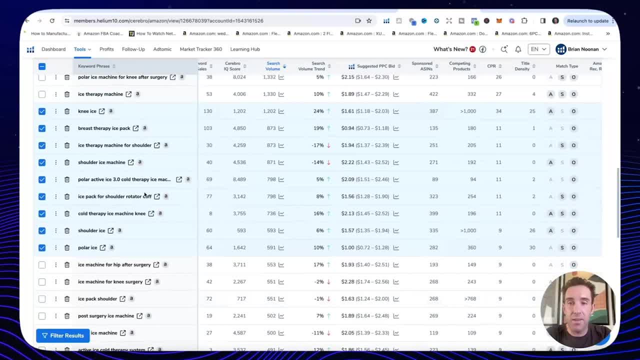 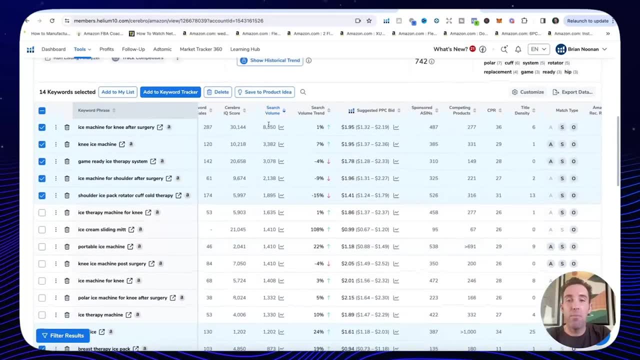 than 5 to 15 keywords per campaign. the reason I did 10 these 10 on on the second broad and second phrase is because they have lower search volume, and the reason I only did five on broad one and phrase one campaign is because they have the higher search volume. all right, and then same. 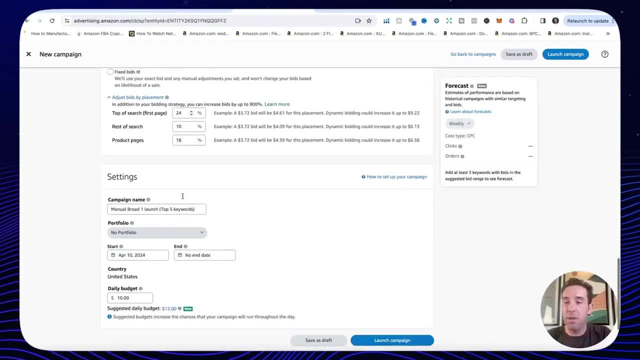 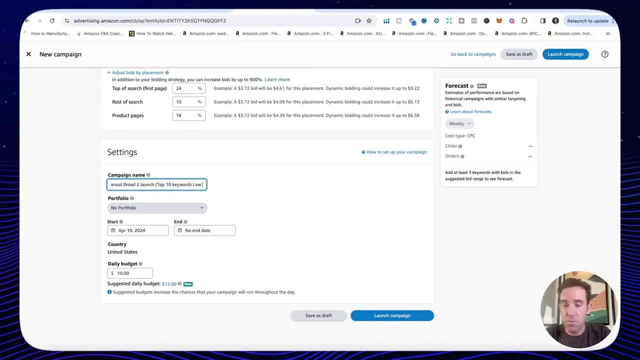 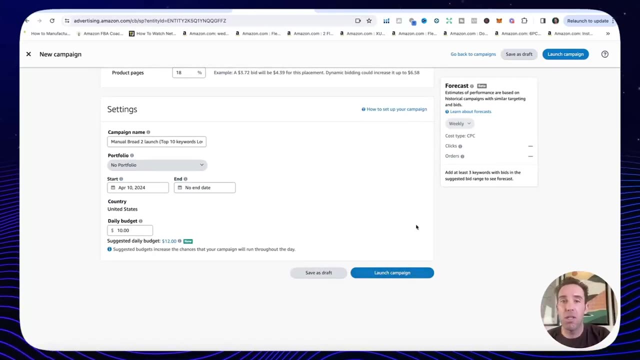 thing down below guys, dynamic bits up and down. you can add a little bit of placements. it's going to be broad. two top 10 keywords- low search volume or lower search volume- runs for four weeks. ten dollar daily budget launch campaign. now we have all of our autos going. we have two broads going. we have two phrase match. 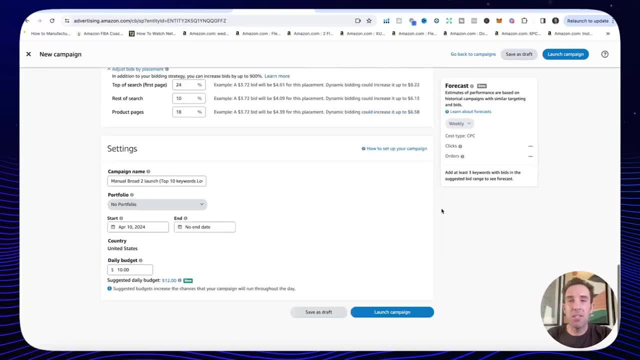 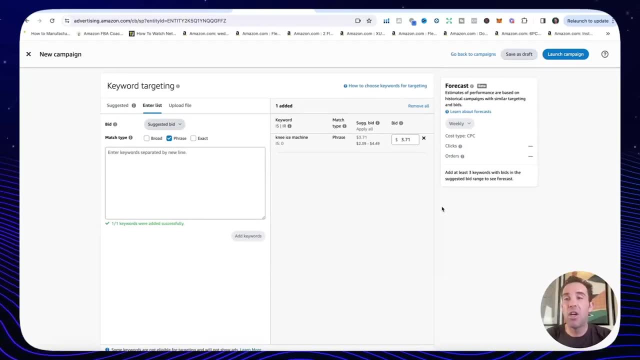 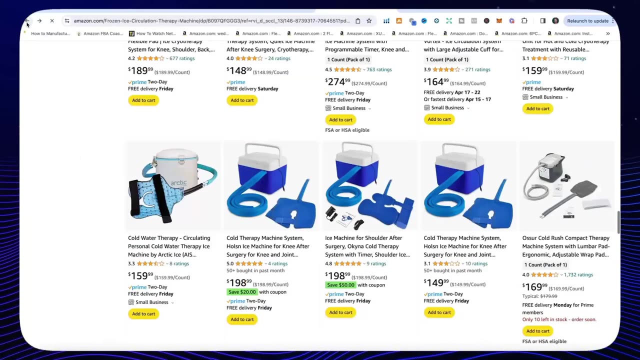 going. let's talk about exact match up next. I would set up exact maps once you have, like, two reviews to your listing. once you have two reviews on your listing, then you can set up exact match just targeting the top three uh keywords that you have in your title. does that make sense? so just do the three keywords that are in your title. so if it's like frozen ice circulation therapy machine, you would Target: uh, maybe ice circulation therapy machine. that'd be the first keyword in my exact match campaign. uh, and then let's say pain: post surgery, cryotherapy for joint pain would be. 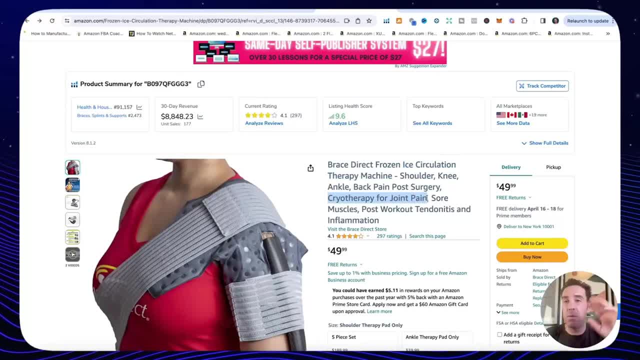 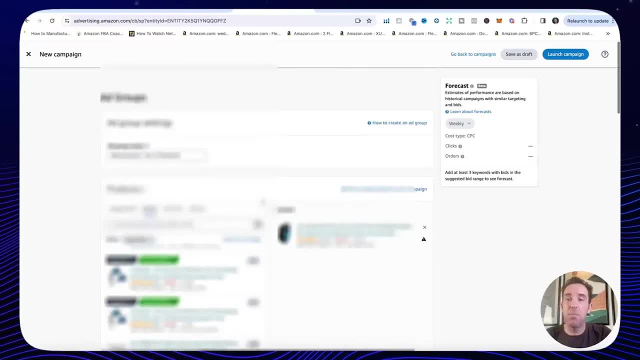 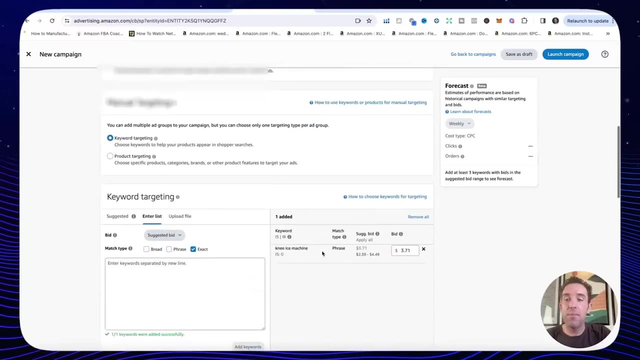 keyword number two. you could put that in the exact match and maybe just run those two keywords in the exact match. let's go over the settings for that. it's going to be at the top the. it's going to be the exact match. top three keywords in my title. add the product, it's manual targeting, it's keyword. 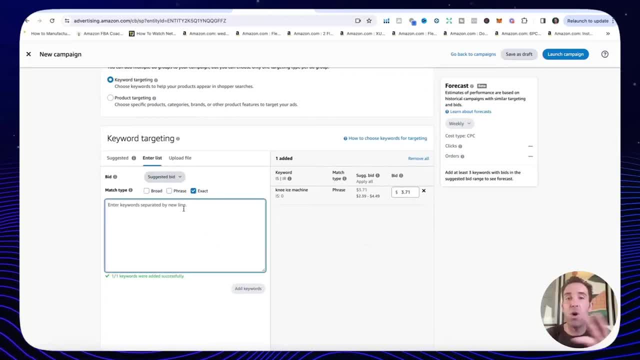 targeting. it's going to be interlist, exact match, just one to three keywords, the top ones in your title. you will have to go higher on your bid here. I would go at least 20 to 50, 20 to 60 cents over the suggested bid. um, ice knee. let me just show you that. okay, so if this, if the suggested is 299, I. 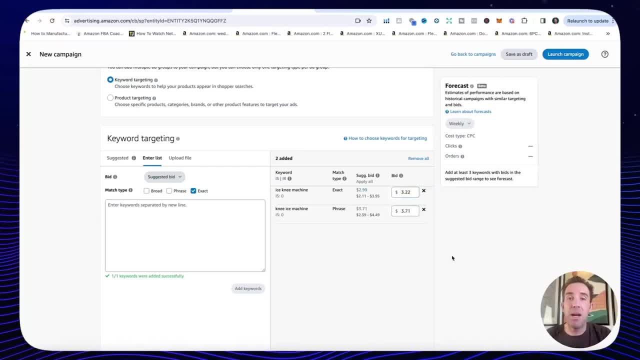 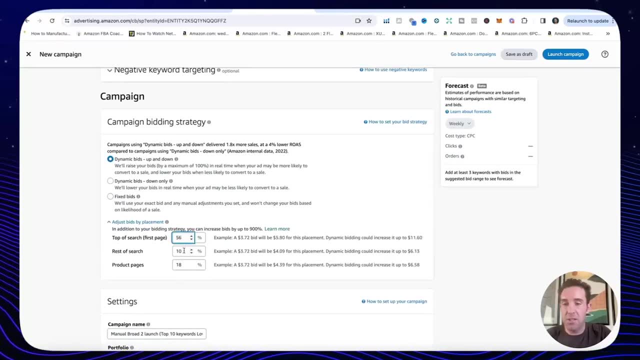 would go like 322 save. uh, because this exact match it's going to be the most expensive, all right, and then dynamic bits up and down. you can go kind of aggressive here on your placements. uh, you're going to need to because it's pretty competitive with having no reviews or low reviews versus all the other competitors who are running. 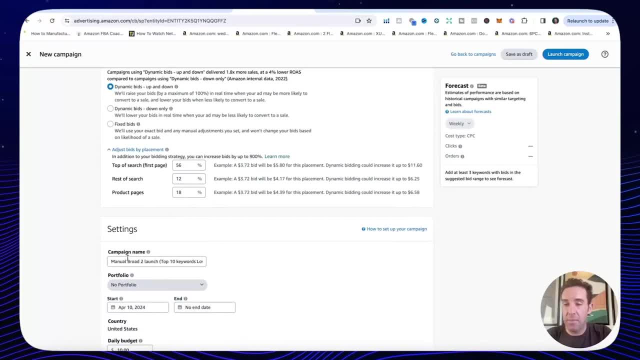 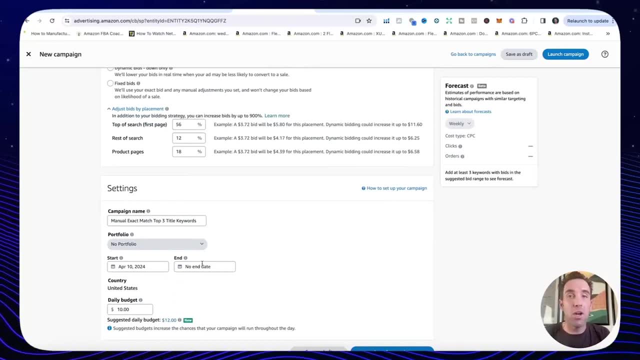 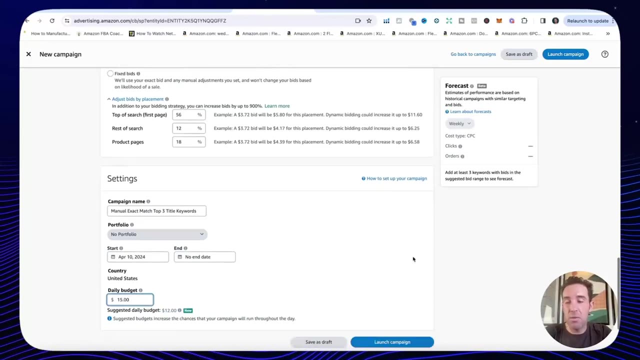 it as exact match. and then this is manual exact match: top three title keywords: this one's only going to run for two, two or four weeks. got to watch this one closely because it'll spend a lot of money and i would do like a 15 budget on this could be 20, 25 and launch campaign. okay, now we 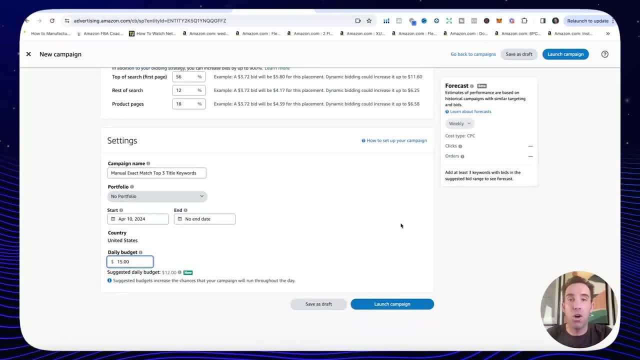 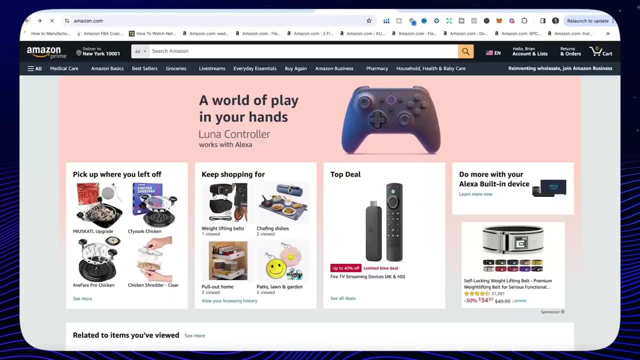 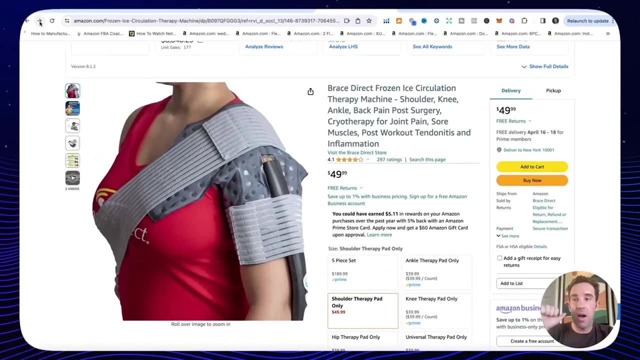 have the exact match going. finally, let me go over product targeting. so if this was my product, um, and let's say i don't have any reviews and i'm at 49.99, you're going to want to pick out guys, some, some, um, some aces of competitors on page one who either have a higher price than you, uh, okay, like. 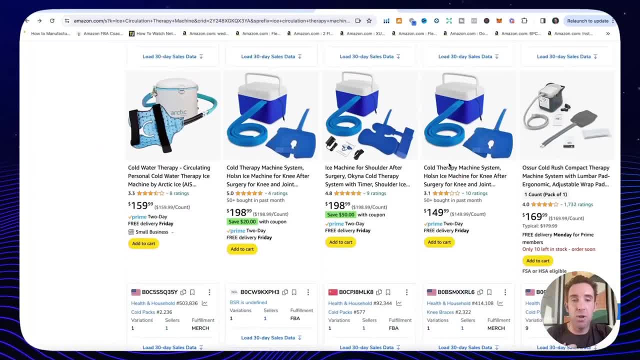 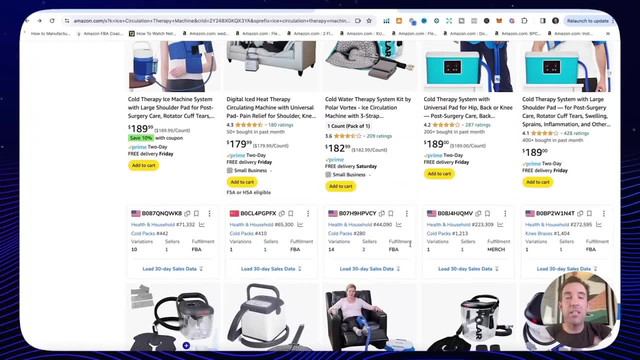 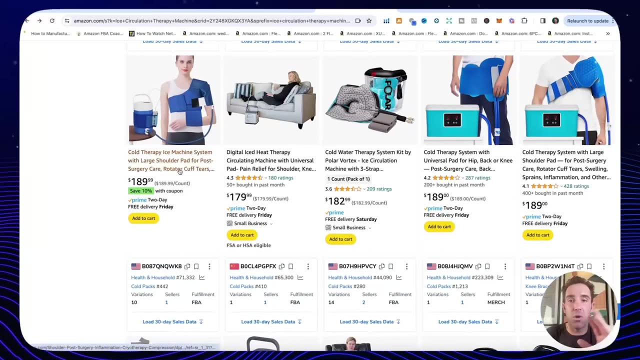 these ones: 198 dollars, mine's only 50, 149, mine's only 50, or, if i have higher reviews, you can target asins with less reviews, or target asins with a higher price, or target ones that don't come with all the features and accessories, as yours does. so so, um, like you can see, like this one looks pretty nice. it i can. 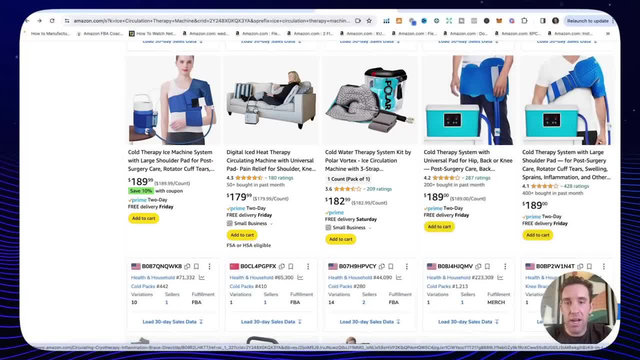 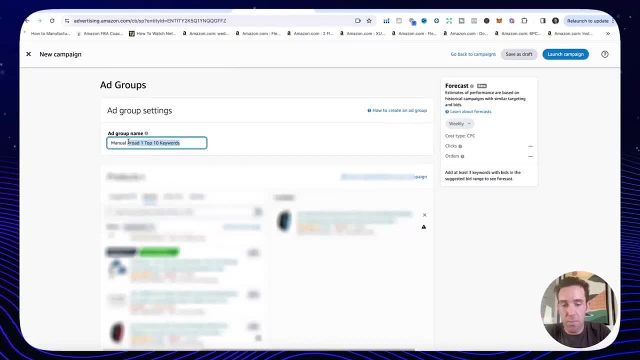 see like three different items here. with this i only see kind of one item, so i would target that ace and mine looks nicer. does that make sense? so let's go over setting up a product targeting. this is going to be manual product targeting top five competitors. okay, we'll add the product that you want to advertise for. 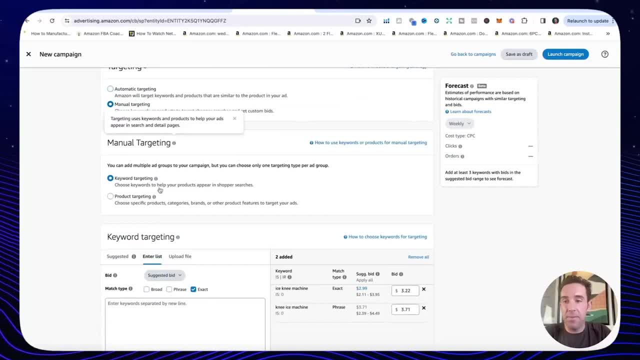 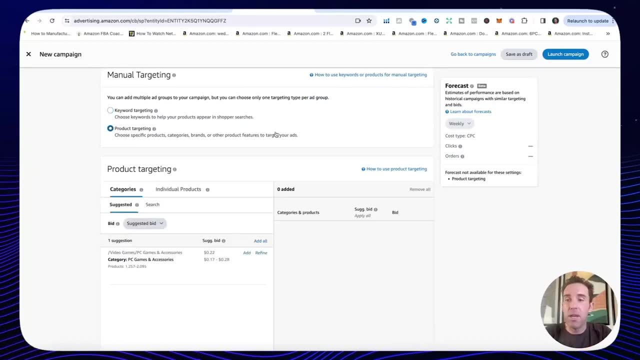 copy this: it's going to be a manual targeting campaign. it's going to be keyword targeting. it's going to be inter- sorry, it's going to be product targeting, not keywords. we're going to do product targeting. it's going to be individual products. it's going to be, uh, inter list, it's. 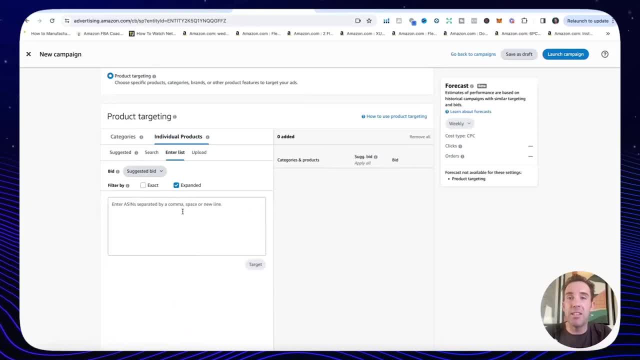 going to be expanded in the beginning. later, once you find some asins that really work well in your auto search terms or even in these ones we're setting up now, then you're going to set up new product targeting campaigns and just select exact, but for now do expand it. that means amazon's. 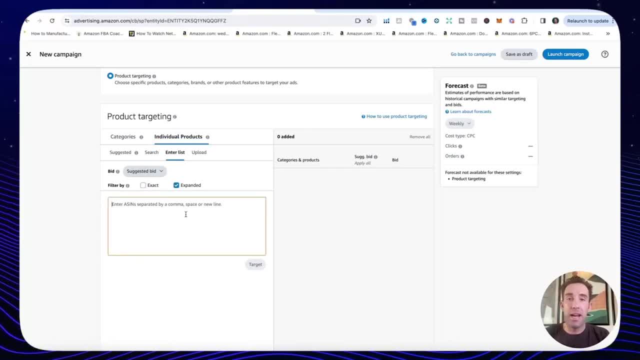 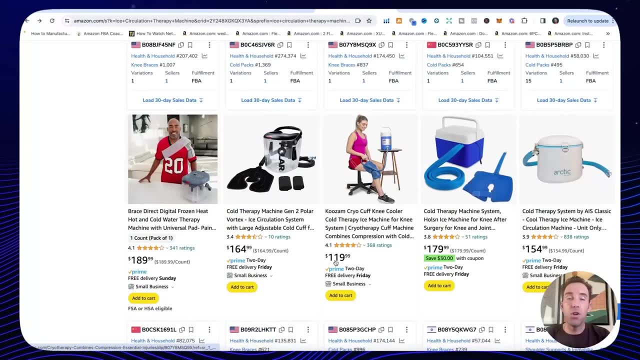 going to show the product actually on other asins that are really similar and that's going to work best- uh, usually in the beginning. so we're going to pick out guys like three to five asins here on page one where you have a good chance- you're you have a good chance of making a sale off of that. 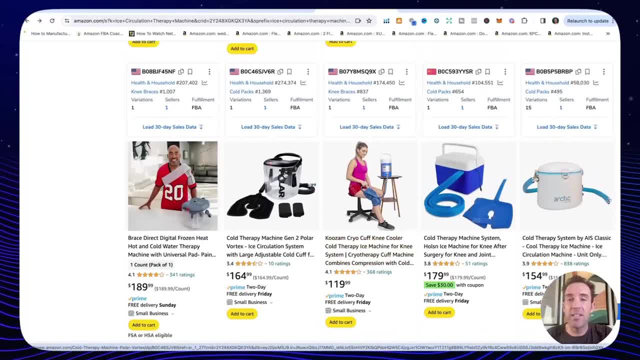 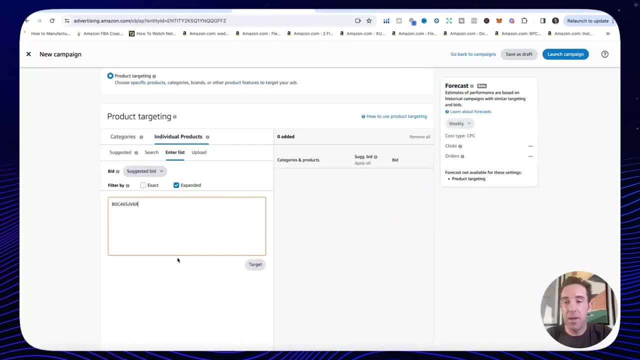 asin. so let's say they have, you know, a higher price, not as much, uh, accessories, not as good. we're going to just click this right here, copy. we're going to come here and paste it there and then click target and then over here, guys, i would go up. so the highest one is 1.78. i would 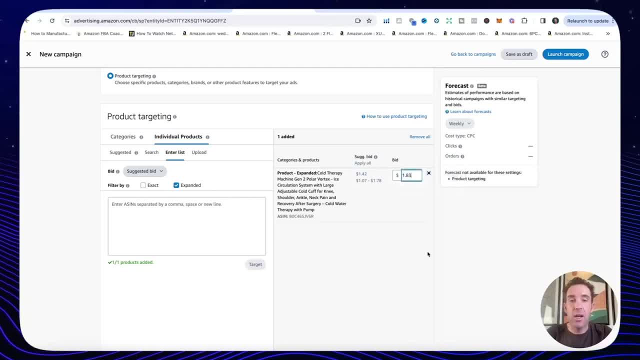 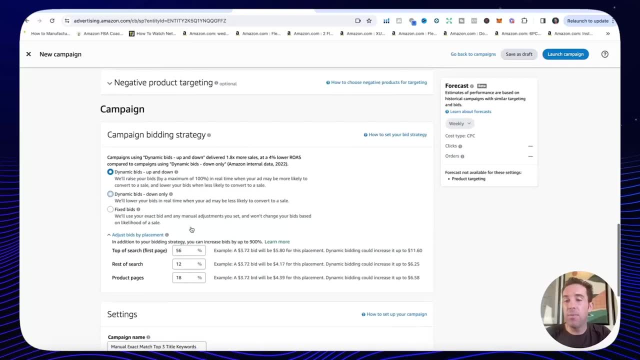 go there, or even slightly higher than that, okay, uh, so we're going like 30, 20, 30 cents over the suggested. then we're going to come down here. it's dynamic bits up and down. we're going to leave these placements kind of where they're at 56. so sorry, top of search is not super relevant here. 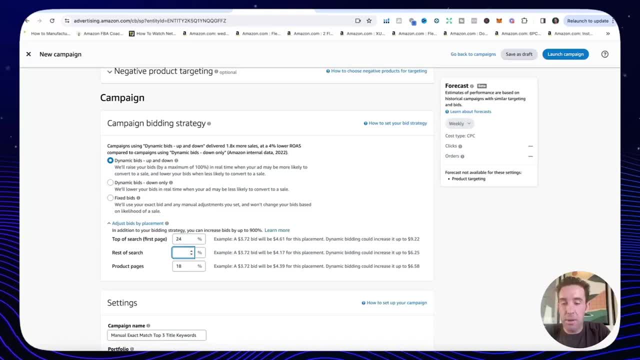 but the rest of these two are. so for rest of search, we're going to go down here and we're going to search. i'd probably go 26 or 46, and then for product pages, yeah, we're going to go 46, 48. you know, i just kind of pick random numbers. but um, rest of search and product pages, this is an asin. 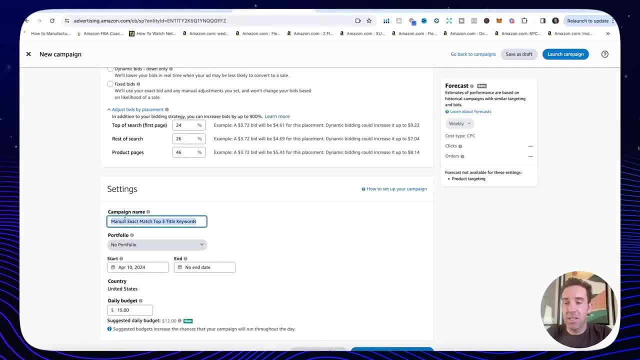 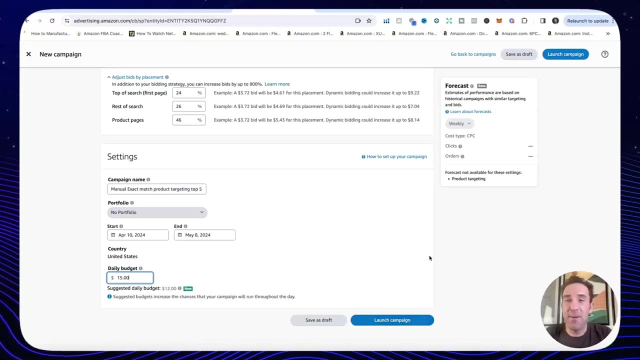 targeting campaign. that's where your ads are going to show. and then this one was not that, it was product targeting, top five asins, okay. and then it's going to run for four weeks, guys, going to be 15 daily budgets. fine launch campaign, all right, guys. that goes over setting up all these. 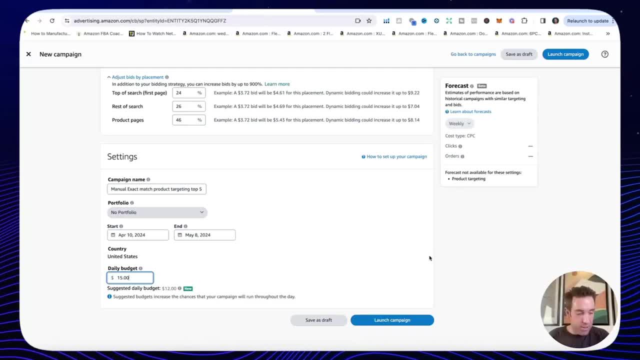 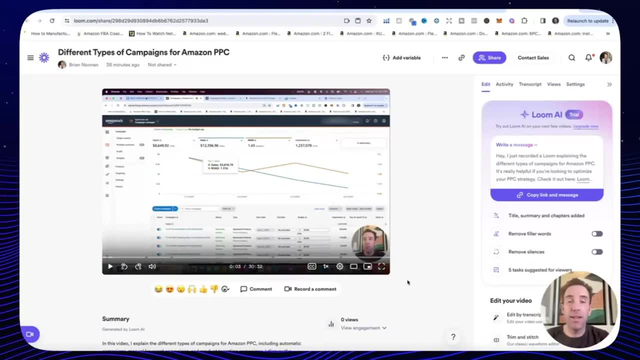 automatic campaigns for launch. oh, this desk has a drawer. i didn't even know that. all right, now that all these campaigns are running- let's say they've been going for two weeks now- how do you come back in? what do you check? how do you optimize? so let's go into there, you're going to come into. 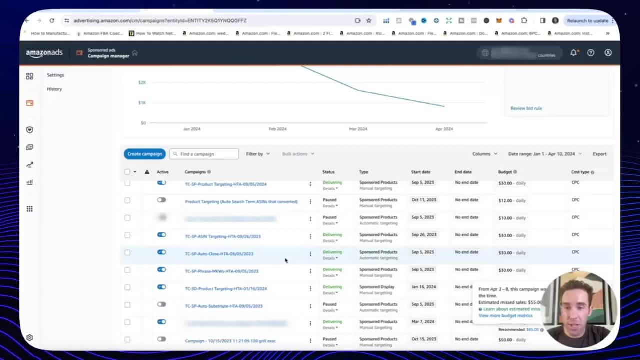 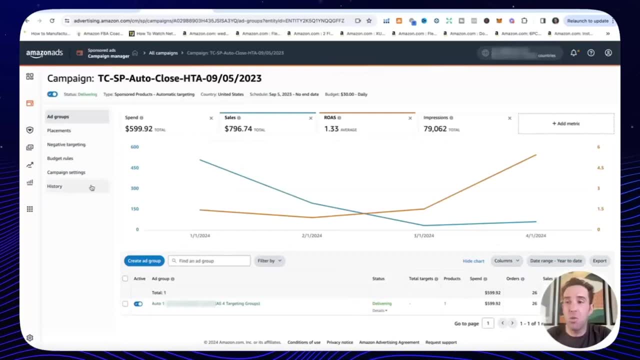 campaign manager, i would work on optimizing the autos first. so let's go here, let's click on an auto first thing you're going to do to optimize the auto after it's been running for at least, let's say you know, one to two weeks. come here, guys. placements gonna click on placements then here. 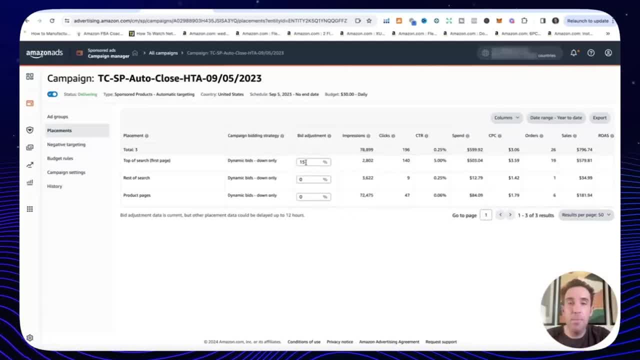 you're going to be able to see those placements and then you're going to be able to see those placement bids. we had set uh, top of search, rest of search product pages where performed best for you. then you'll adjust these on each campaign. okay, so here you can see. top of search impressions is. 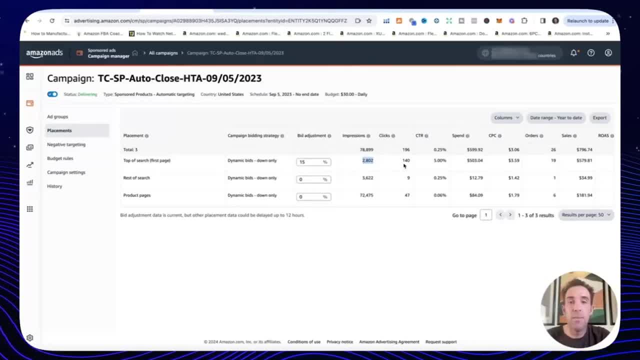 pretty strong: 2 800 customers saw the ad. 140 140 customers clicked on the ad. that's a ctr of five percent. that's good. 503 dollars in spend. cost per click is high: 19 orders, 579 dollars in sales. so in this case- i've already brought this down, but you could see this one was probably at the 50 or 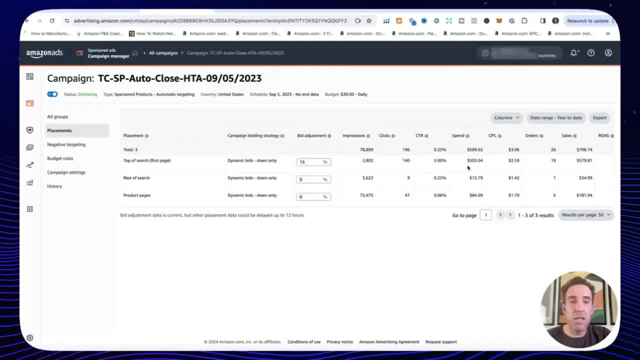 60 or higher level. i brought it down to 15 because we're trying to decrease the spend for the sale next up, rest of search. i think i had probably 18 or 14 uh set here. you can see um 3 600 customers saw the ad. nine customers clicked on the ad in the rest of the search placement area. that's. 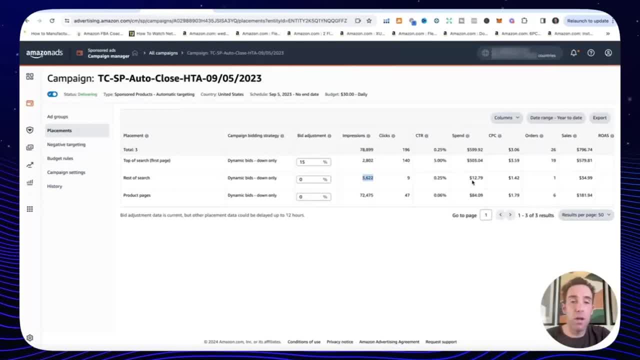 his click-through rate under one percent. not good. twelve dollars in spin for one sale. i would decrease that five or ten down. finally, product pages: 72 000 customers saw the ad. 47 customers clicked on the ad. the ctr is nowhere near one percent or higher. spent 84 dollars, but i did make. 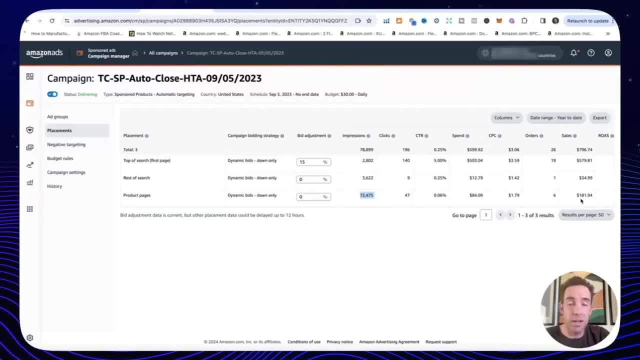 six sales, or 181 in uh sale sales for 84 and spend. so if this was at like a 26, i would actually consider increasing this. even though the ctr isn't good, the spend is much lower than the sales. so if this was at 22, 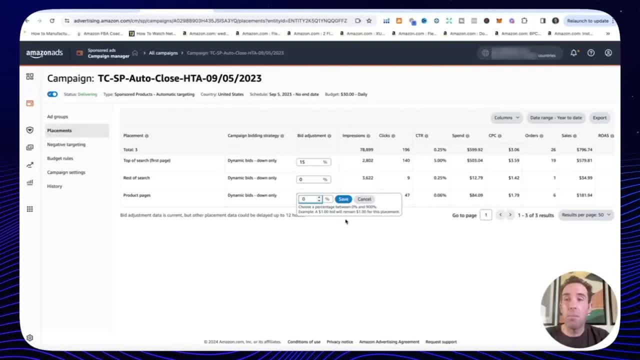 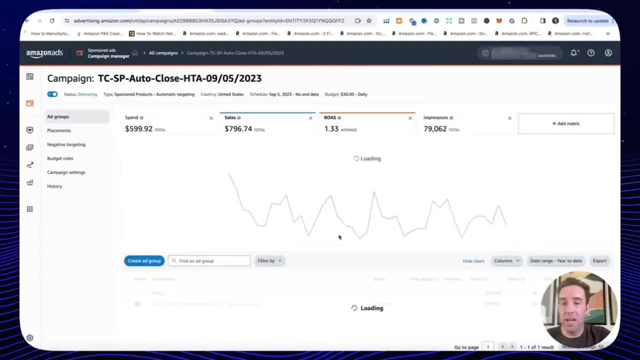 or 26. i would go up maybe five or six, uh points, okay. uh, the other ones came down, though, because the spend is quite high for the amount of sales you made. then you're going to go back here. this is an auto campaign. you're going to click on the targeting group name right there. then you're 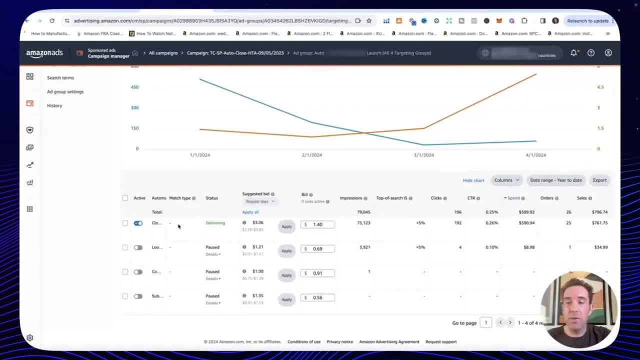 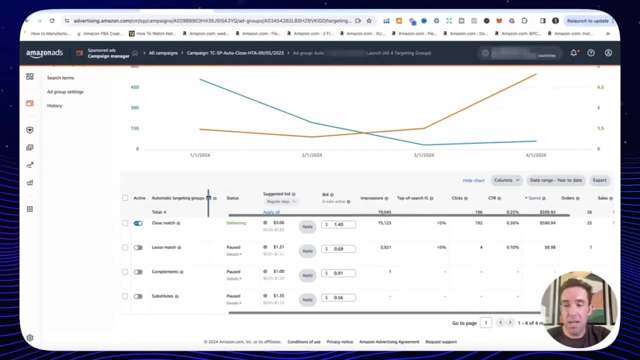 going to come here. click on targeting and then you can see here you have the four targeting groups and you'll have data here. you'll need to adjust these targeting group bids first, up close match. how'd it do? 75 000 customers saw the ad- 192 customers. 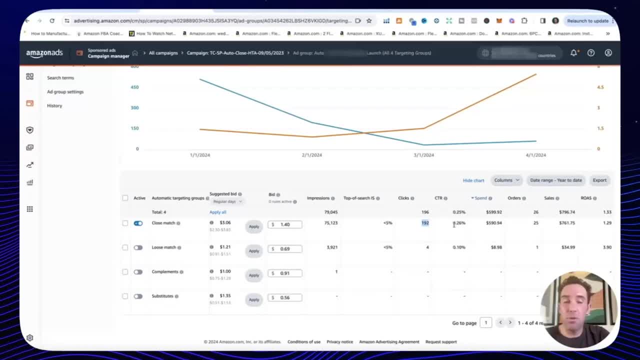 clicked on the ad. the ctr is not, uh, one percent or higher. not, it's uh quite low: 590 and spend: for 25 orders, 761 in sales. i would actually bring this down, um, about 10 to 20 cents down. we're trying to decrease the spend for the amount of sales you made. you're going to have quite low. 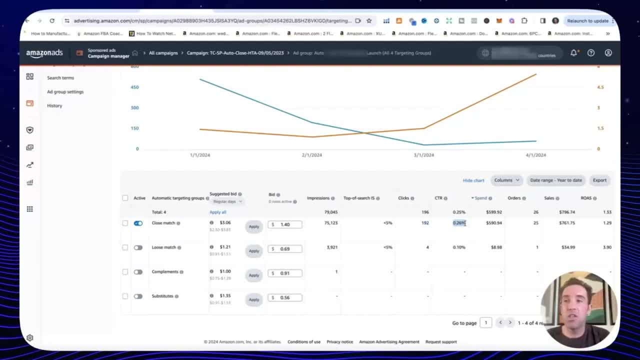 ctr in the beginning, like this oftentimes, guys, as you're just trying to test different main images, maybe different price points that work well, but those are the main things that affect ctr. click through rate, main image, price, title and reviews. once you have some reviews, your ctr will also. 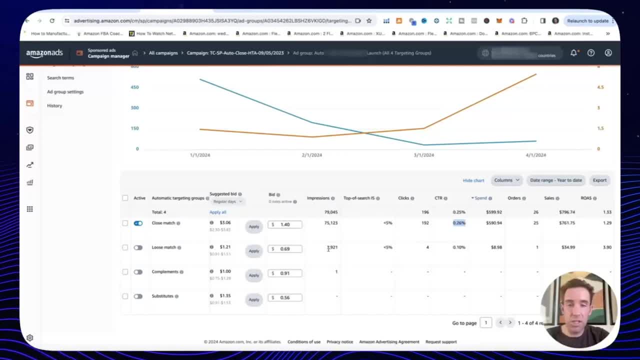 increase here. uh, loose match. section 3: 900 customers saw the ad. four customers clicked on the ad. i spent eight dollars and i made one sale. i would probably just reset that bid. if it's at 69, i would probably just reset it to 0.71 or 0.73, just because i like that it brought one. 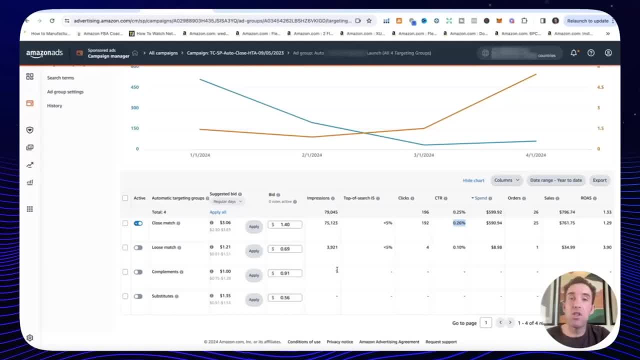 sale these other two compliments and substitutes. you can see there's no impressions at all, or one and nothing. in that case you're going to have to increase the bid up. this is before your auto one: all four targeting groups. you'd want to increase that five or ten uh cents higher to try to get some. 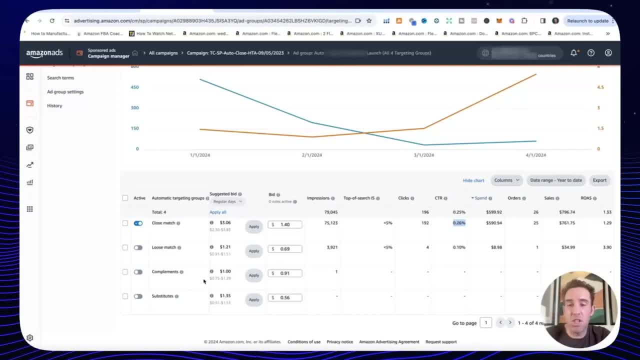 impressions. um, if this is uh same thing, if it was just one of the one ad groups turned on, if i just had uh compliments on, you'd want to still increase it. try to get some impressions. then you're going to come to search terms. guys, you're going to come here. i like to sort this first high to low by spin. 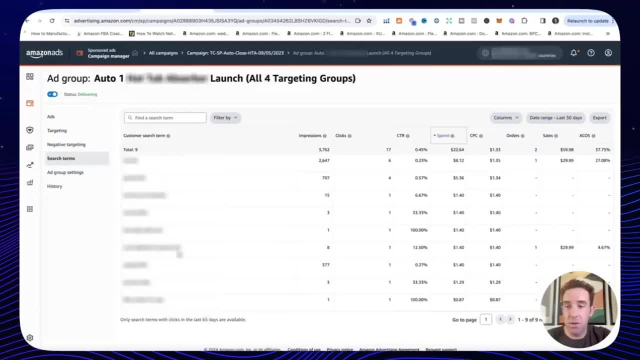 for a new product launch and you're going to go into your search terms here and this is going to show you all the keywords and asins that amazon showed your product for, and which keywords and asins brought you sales and which ones you need to shut off. so this one, this first keyword, brought a. 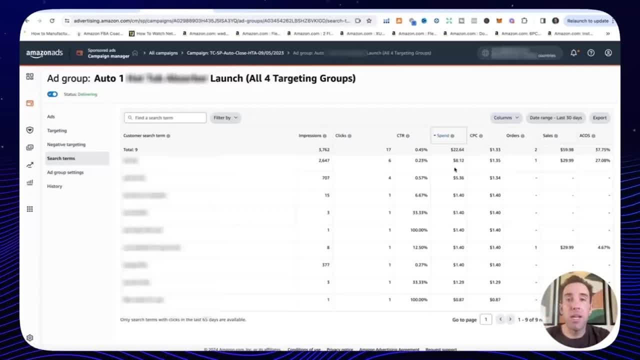 sale for eight dollars. what do you do with that? i would keep it running in here. i'd also make sure i move it or it's running in my broad and my phrase campaigns. if it continues to perform super well in here, i would add it to an exact match campaign. you will not compete against yourself, guys, if you're. 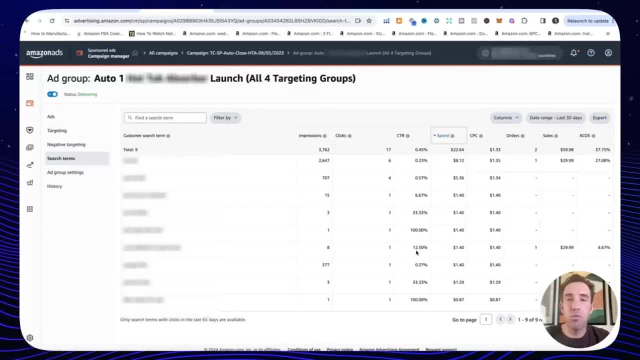 running this keyword in here as auto and you're also running it as broad, or you accidentally put this keyword in broad, uh, two times. amazon has stated that as long as you're running from the same seller account, you will not compete against yourself on keywords. okay, and then this: so we're. 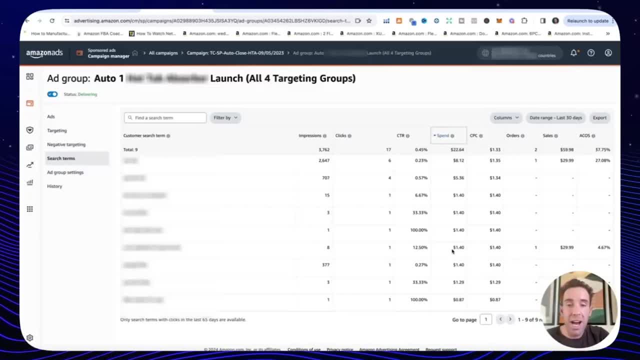 looking for. this is another one right here. guys, you're going to want to make sure that you're running it as broad as you can see here this keyword. i made a sale for 1.40. i would want to make sure i keep that one running in here. it's working, and i'd also want to make sure i'm running. 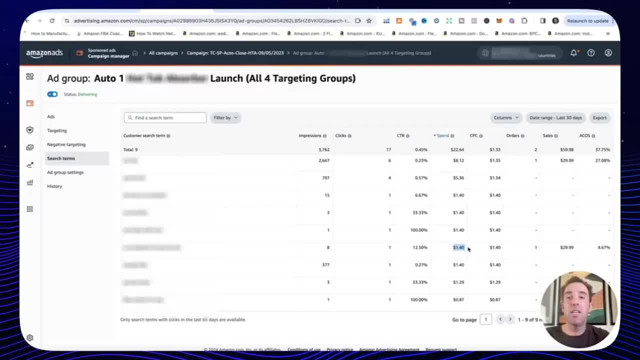 that in my broad and my phrase, and possibly in my exact match, to continue testing and figure out where it works best and then optimize from there. and then, finally, guys, we're looking for any keywords or asins wasting money. this one's getting close. the ctr is not over one percent, it's already. 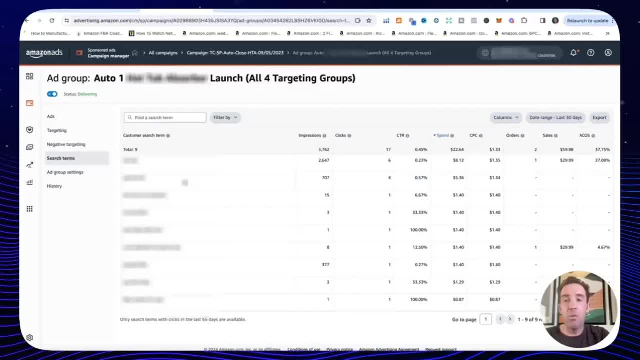 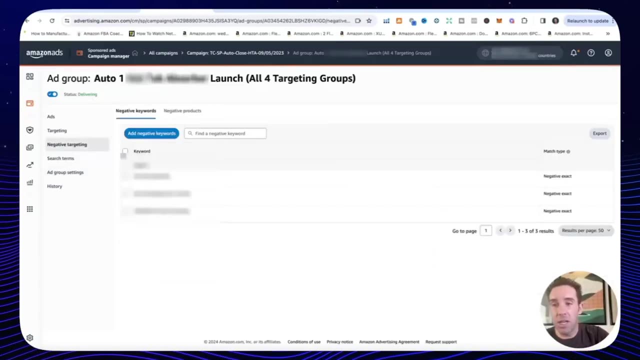 got four clicks, it spent almost six dollars and brought no sales. how would you shut that off? you're gonna copy the keyword. if it's got like 10 clicks or more or 10 in spend or more and a low ctr, copy it the keyword or the asin. come over here to negative targeting. 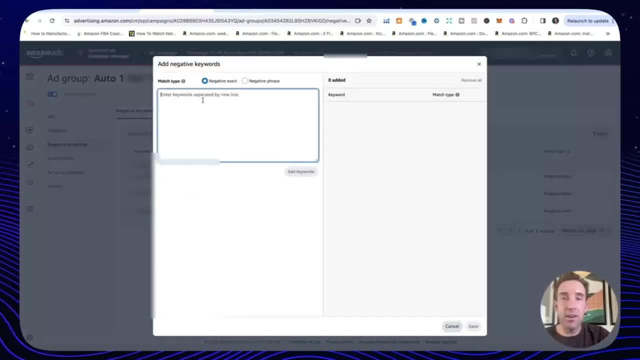 click on add negative keywords, paste it here as always negative exact- and click add keyword and save. and now you've just told amazon i don't want to waste any more money on that keyword. it had 10 or more clicks or 10 or more. spend low ctr, way under one percent, and i want to shut that off. okay, so you'll stop wasting money on that. 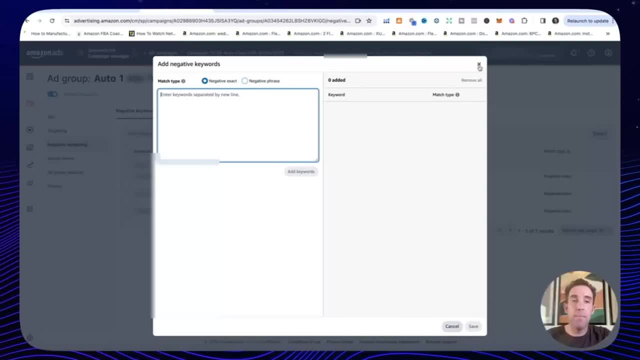 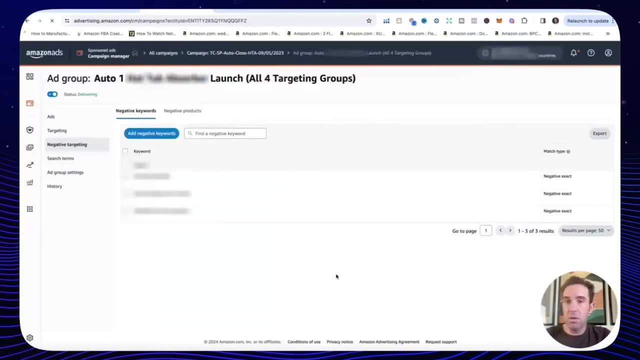 always negative exact guys. okay, don't do negative phrase um, because that will shut off any keywords related to that one. so that's how you're going to optimize your auto for a manual campaign. it's similar, a little bit different, so you'll click on the manual campaign from campaign. 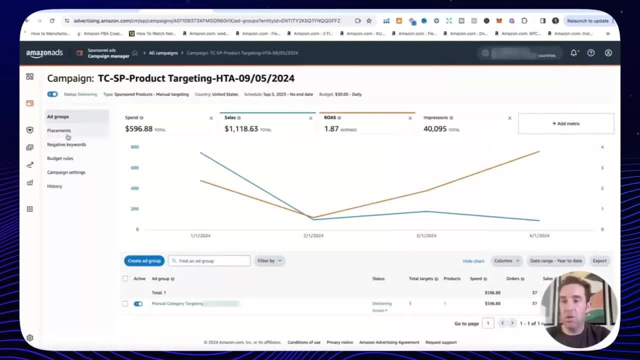 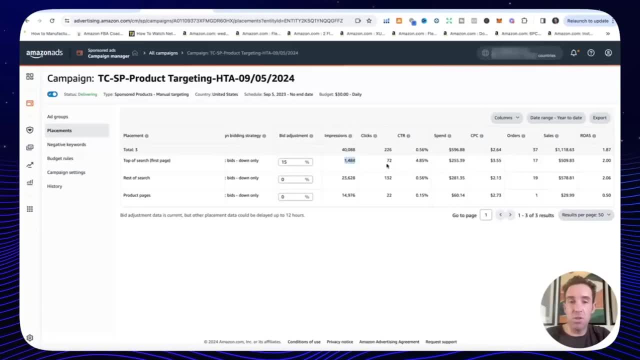 manager: uh, let's, i'll show you a product targeting one. you'll go to placements. same thing. we're going to adjust the placements based off how it's doing here. 1 400 customers saw the ad. two customers clicked. almost five percent ctr, that's good- 255 and spin for 509 in sales. i would. 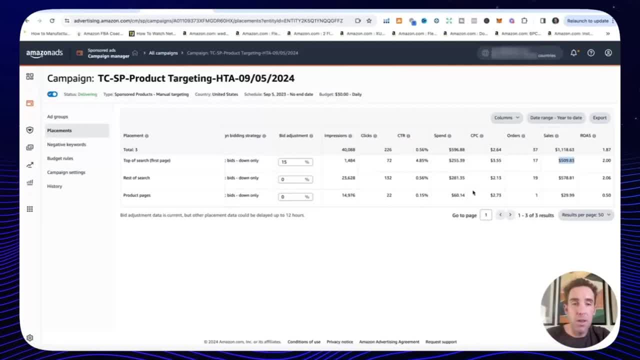 leave this placement where it's at or even increase it five. this one, i'd also increase it 281 and spin for 578 sales. i'd increase it five or ten, this one 60 and spin for only one order. go down. i would go down 10 or 20 percent on that placement. then come over here to ad groups, come. 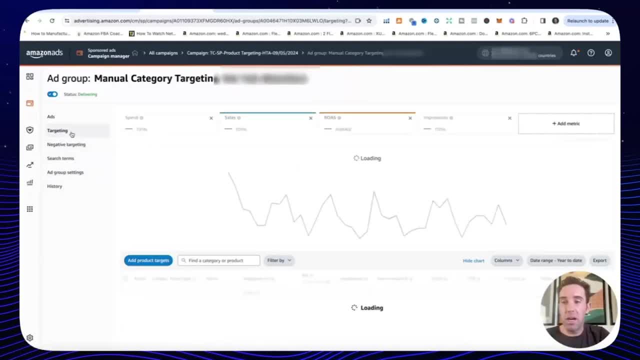 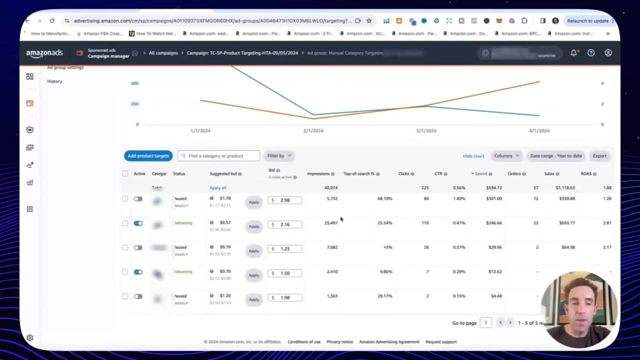 down here. click on the ad group name, go to targeting on the left side side and you're going to want to adjust your bids on the keywords or asins themselves by looking at the data. first up 301 and spin for 359 in sales. i would bring this bid down. 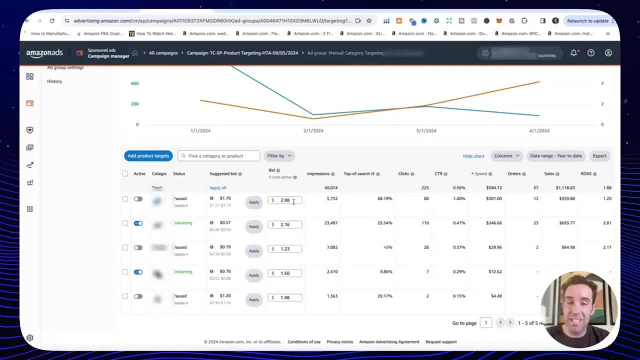 like 2.88, 2.66, 68. bring it down 10 or 20 cents, keep it running. next up 246 and spin for 693 in sales. ctr is kind of low, uh, but i would increase that five or ten cents up next one thirty. 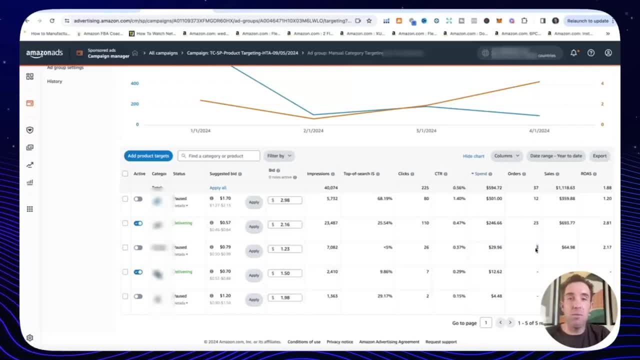 dollars in spend for only two sales. we could not spend fifteen dollars a sale. i would decrease that five or ten cents. this one, seven clicks twelve dollars in spend, a very low ctr. that one is wasting money. i would switch it off or just start by cutting it by thirty to fifty percent. let it go. 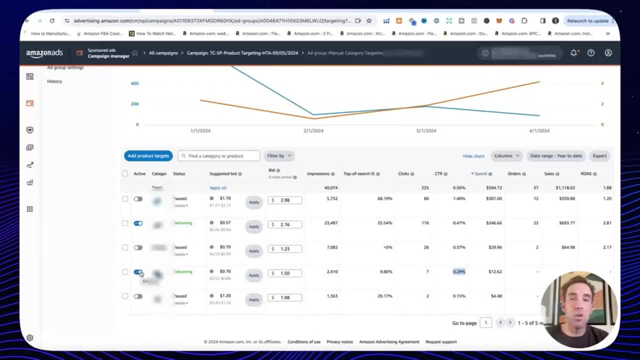 for another week or two. if it doesn't generate a sale at the lower one, then you can switch it off entirely. okay guys, that's gonna be how you go in and optimize your autos and your manuals after they've been running for two to four weeks. i hope you enjoyed this video going over amazon pbc: uh, in-depth tutorial. i look.